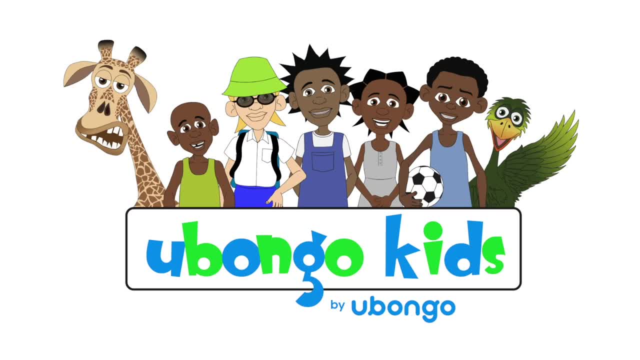 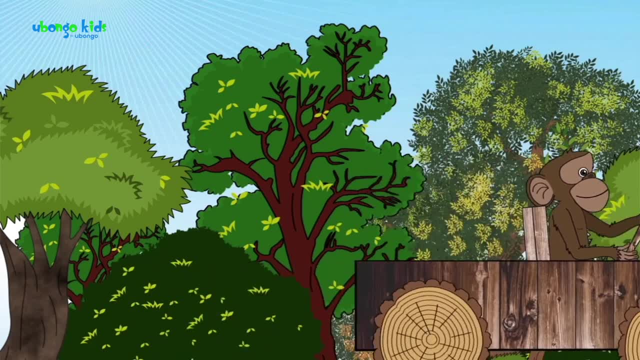 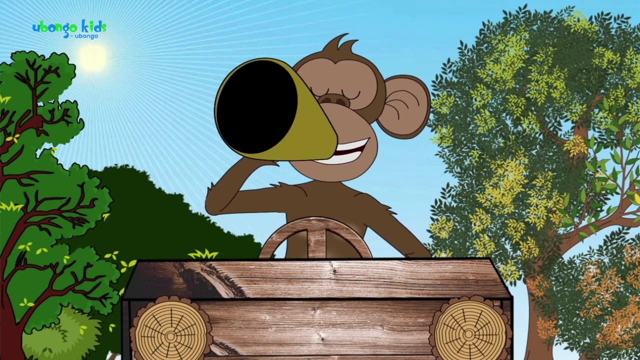 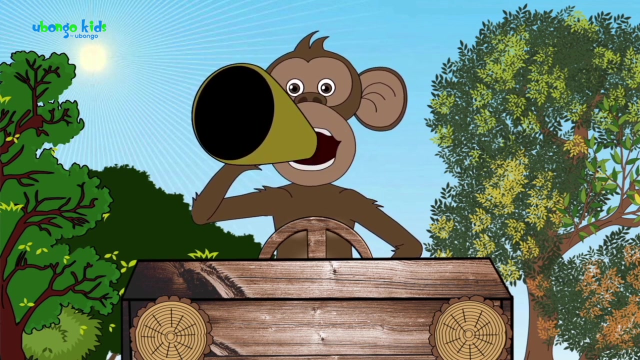 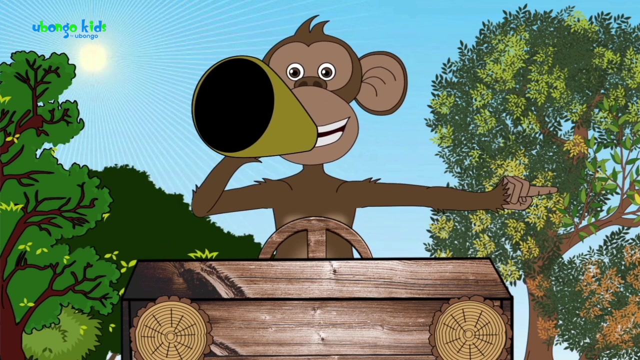 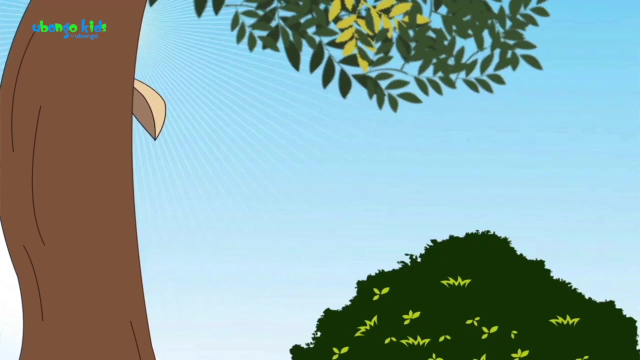 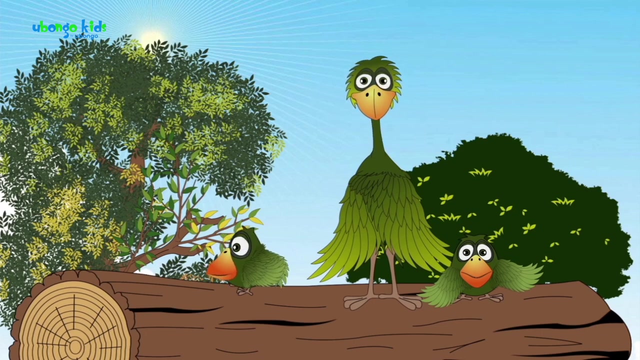 Attention, Attention. There will be a singing competition for the animals of Kokotoa. Come and compete Tomorrow. there will be a free bus at 11 am from the Seven Mangoes bus stand. Be there or be square. Ma'am, I'm in. 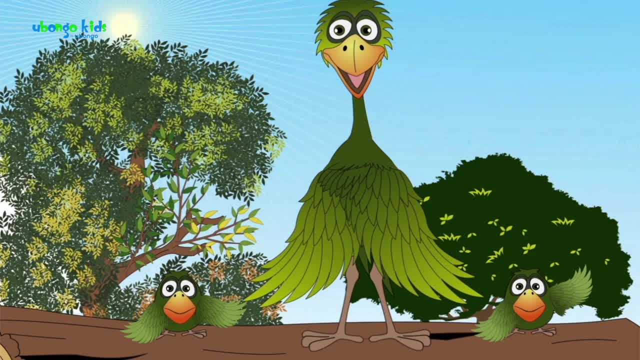 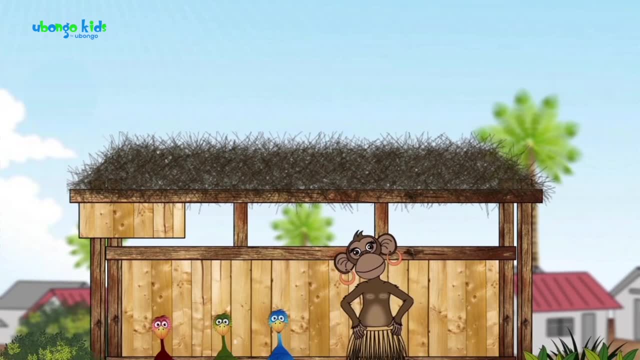 I'm in too, and I'm gonna win. Last year I didn't win, but this year I've been practicing all year long and I have the perfect song. Wait till you hear it. It's gonna be the best song there. Everyone's gonna be so proud of me. 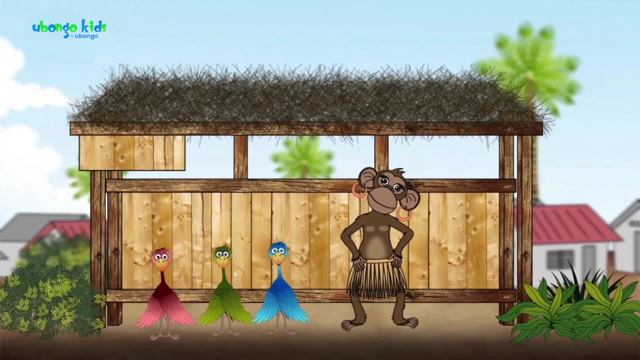 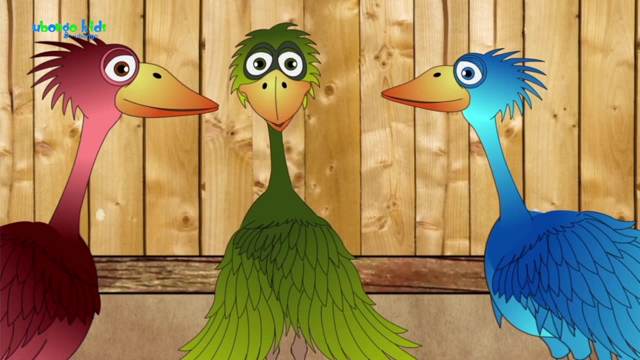 What is this I-I stuff To say: we, not you? Oh yeah, we've been practicing all year. Last year we didn't do that well, but this year we have the best song. Are you all going to the singing competition? You might as well all go back home. Don't waste your time. 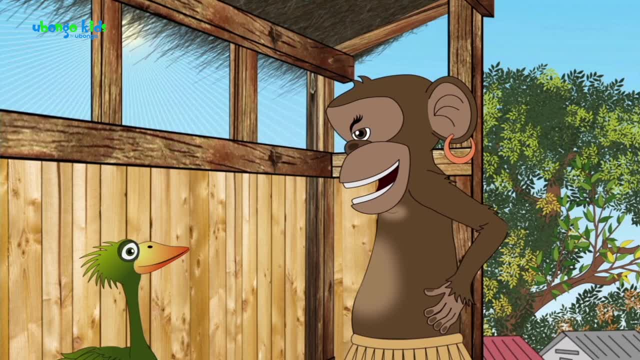 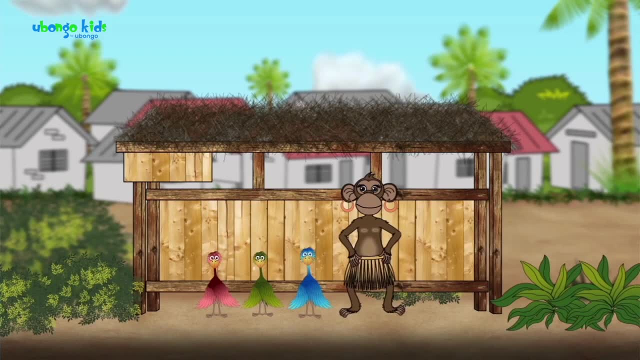 The winner is me. The winner is right here. Just you wait, Mamandege. The winner will be known soon enough, and it won't be you- Definitely not you. You'll see What is this I-I stuff. It's gonna be the best song there. Everyone's gonna be so proud of me. 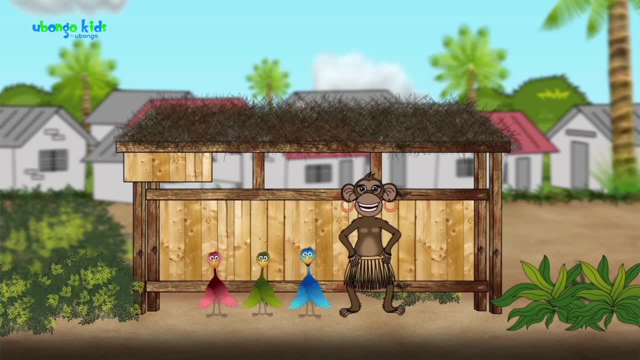 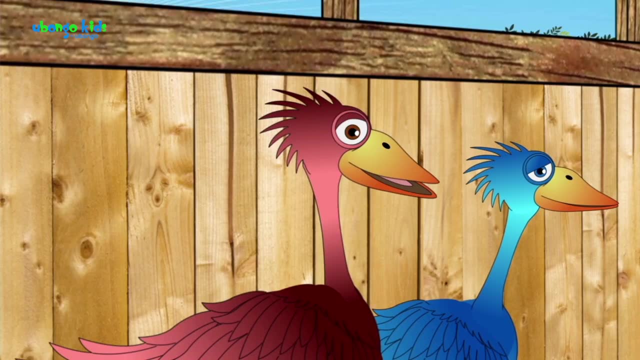 The day before yesterday I went there and there were so many people. Now, where's this bus, Patience sister? Right now it's just 9 o'clock And they say the bus will be leaving at 11.. So just hold your horses and wait till it's time, eh. 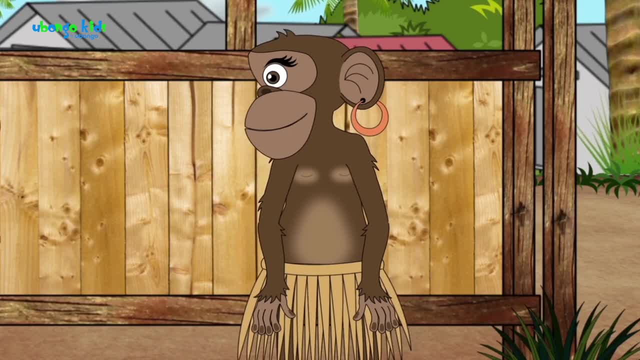 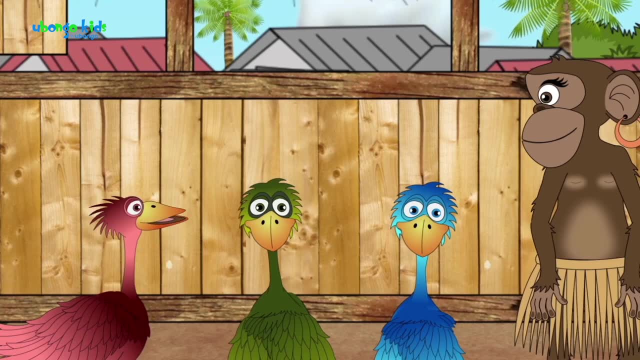 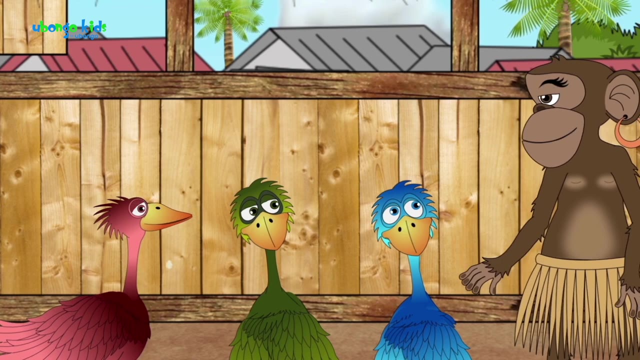 Are you with me? I'm so excited, Man. we've all gotta wait until 11?. That's so long. What are we going to do? It's not that long. How many hours are left until the car gets here? Hmm, Let me calculate it. 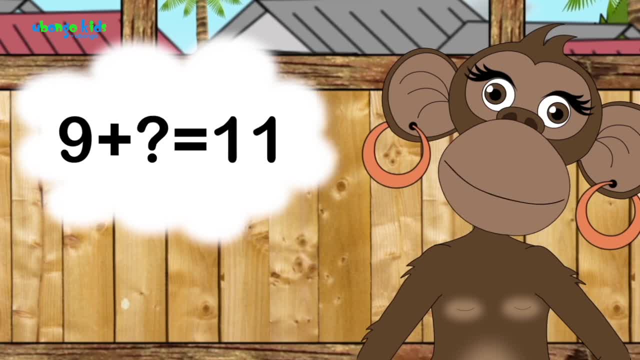 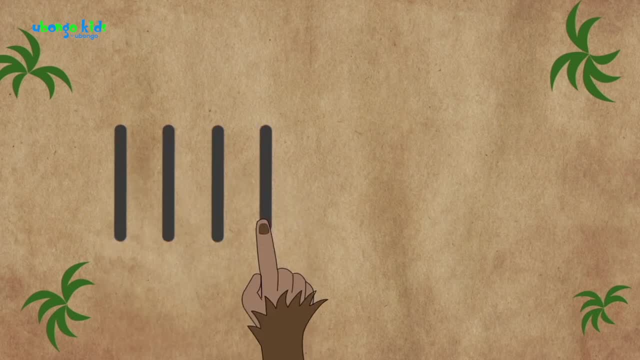 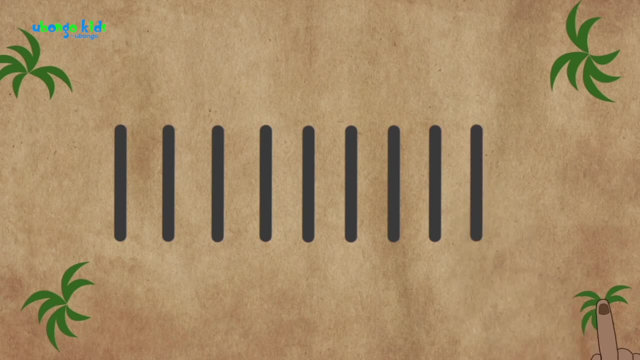 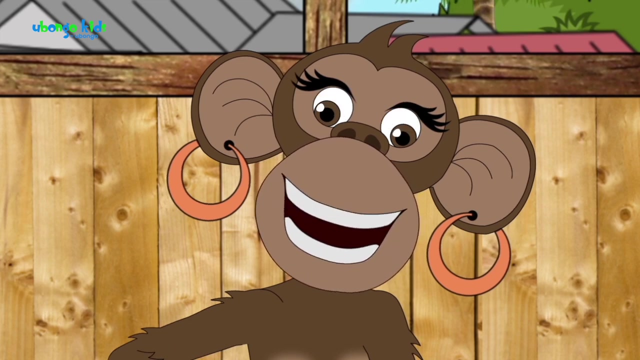 9 plus what equals 11? So let's start with 9.. I'll draw them like this: To get to 11 o'clock, I need to draw two more lines. So before I add more lines, let's count up the ones we've already drawn to make sure we've had the right amount. 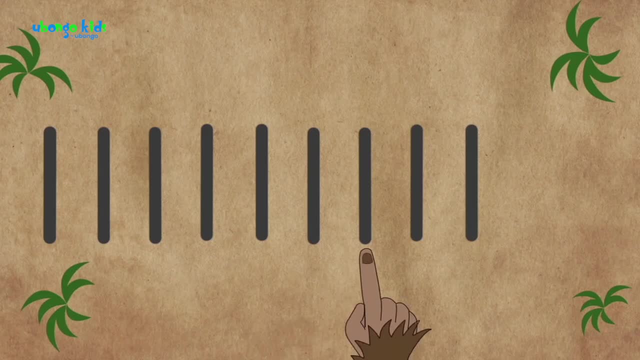 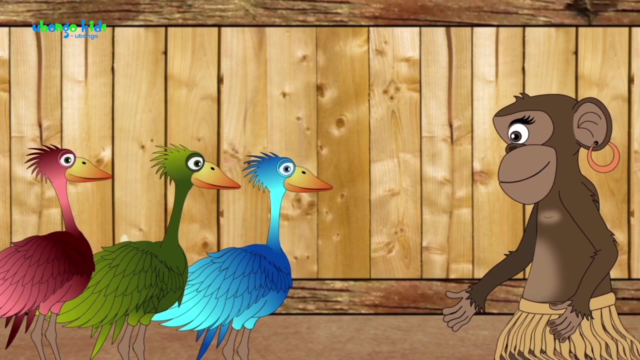 7, 8, 9, 9 plus 9 plus 10, 9 plus 10, 9 plus 10, 11, 11, Uh-huh. You see what I've done now. You guys see I don't get it. You see what I've done now. You guys see I don't get it. 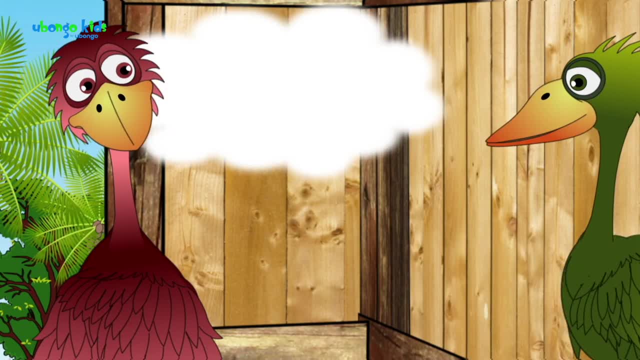 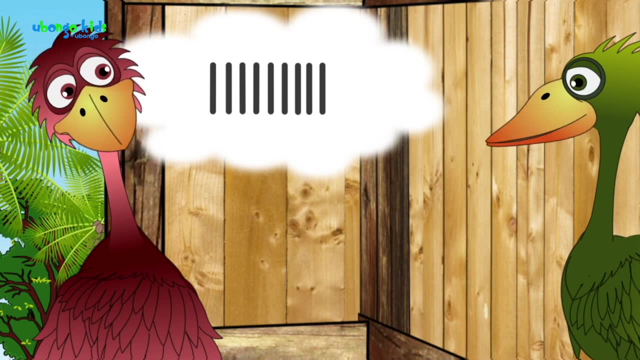 Come on, guys, That is so easy. Now look here: We already had nine lines, So to get up to 11 lines, we needed to draw two more lines. You see, That is so simple, right? So to get up to 11 lines, we needed to draw two more lines. You see, That is so simple, right. 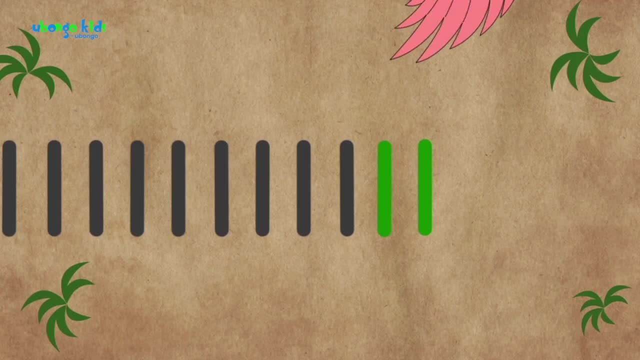 So to get up to 11 lines, we needed to draw two more lines. You see, That is so simple, right? One, two, I get it now. You've added two lines. One, two, I get it now. You've added two lines. 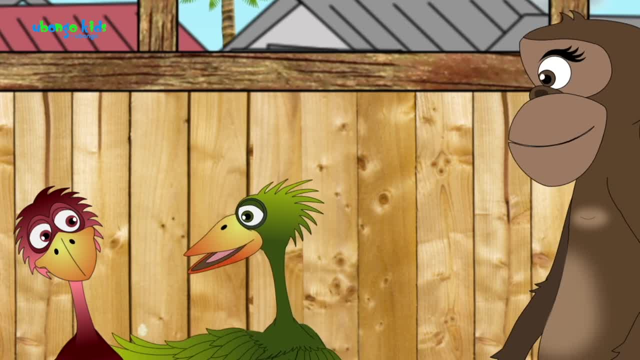 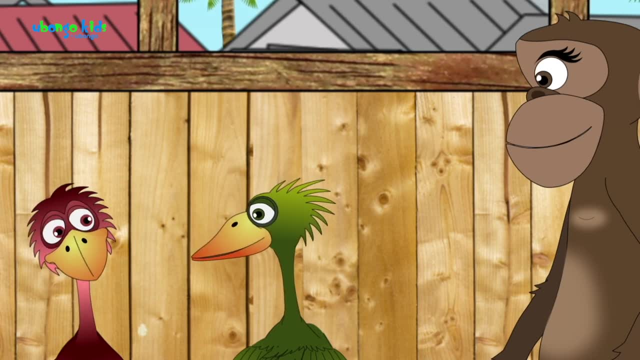 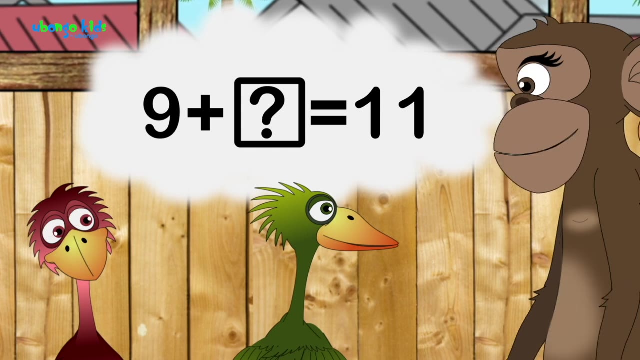 So we can say that to get from 9 to 11, we need to add two, So we have two more hours until 11 o'clock. It's just like saying 9 plus how much equals 11, right, There you go. So it's 9 plus how much. 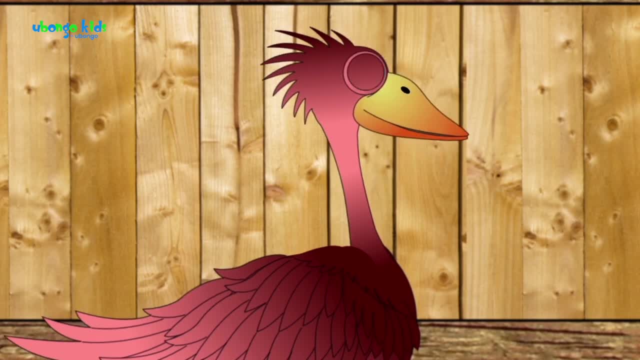 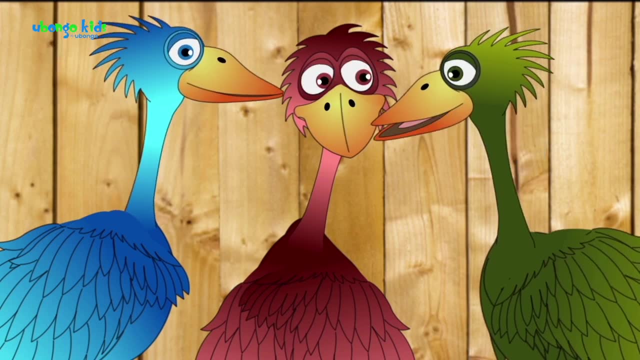 There you go. So it's 9 plus how much? Well, that's easy, It's 9 plus 2.. Well done, What a clever girl. So since it is 9 o'clock now, we need to wait two more hours, until 11 o'clock. 9 plus how much will give you 11?. 9 plus how much will give you 11?. 9 plus 2 will give you 11.. 9 plus 2 will give you 11.. 9 plus 2 will give you 11.. 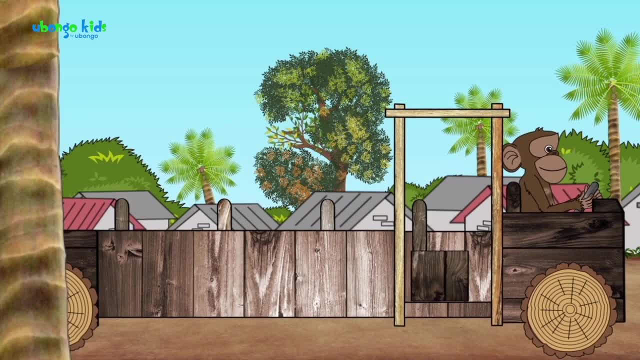 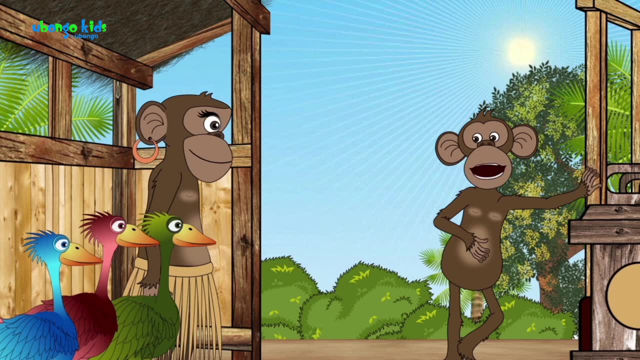 That's good. That's good. Good afternoon. My name is Gadare and I'm your bus conductor for today, And I'd like to welcome you aboard Gadare Bus Services, heading for the Magic Mouth Music Competition, And for one day only. you get on for free and get off for free, OK. 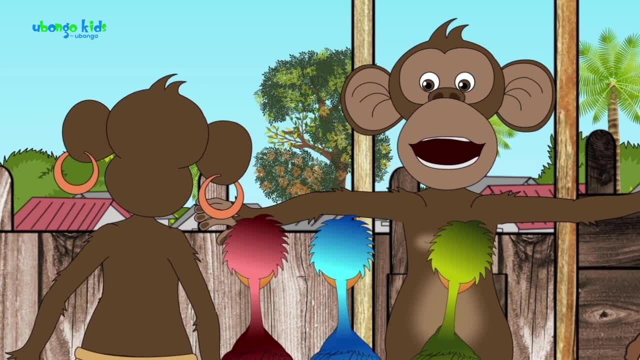 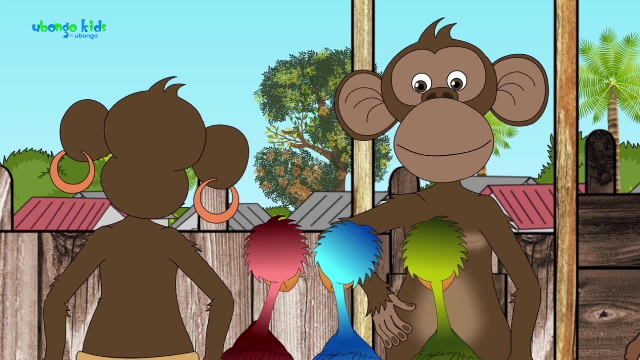 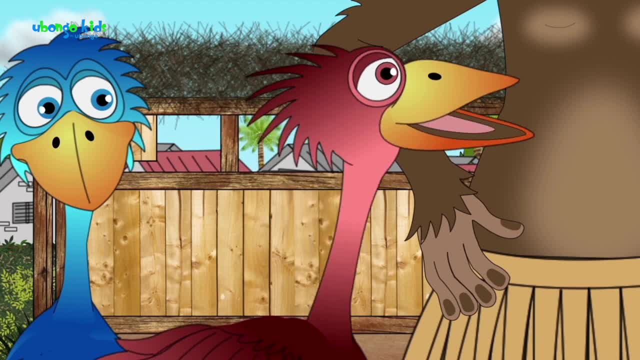 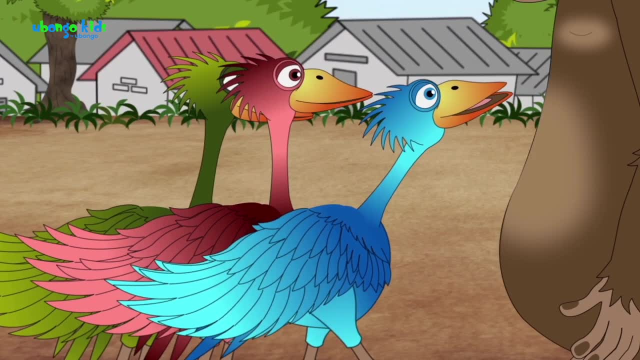 camp. What kind of conductor are you And you're calling yourself a conductor? Get out the way and let me conduct this bus. And why are you looking at me like that? You've never seen a bird conducting a bus. Why are we waiting? I've been on a bus before. I don't need instructions from you about. 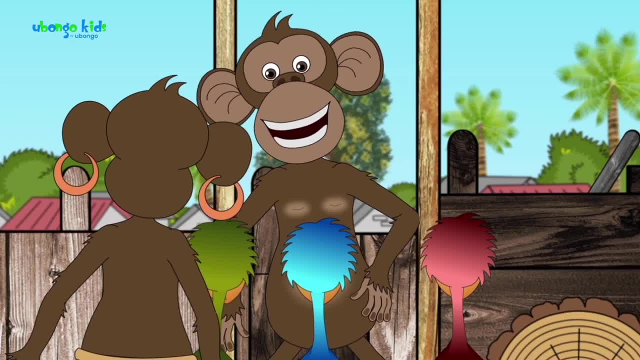 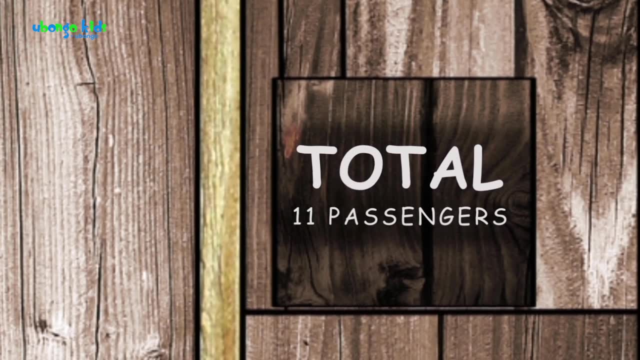 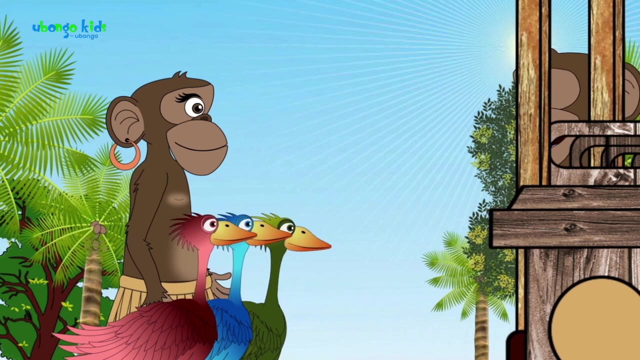 how to get on a bus. We've been standing here for ages And you will stand here a lot longer if you keep that up Now. this bus carries 11 people, so we are not leaving here until there is 11 people With room left for me, of course, because I've got to drive. But even with me and the few of you, 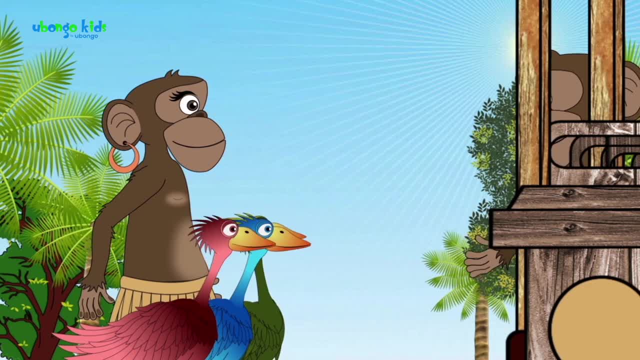 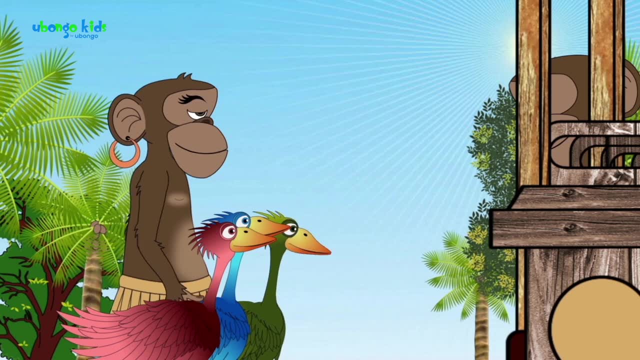 there's no way we'll fill all those seats, Gedere, come on now. Clever as you are, you haven't managed to calculate how many more passengers are needed to fill the seats. Gedere, listen, let's climb up the tree and I'll show you. 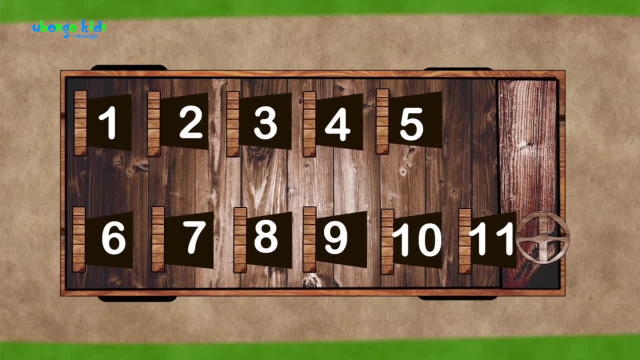 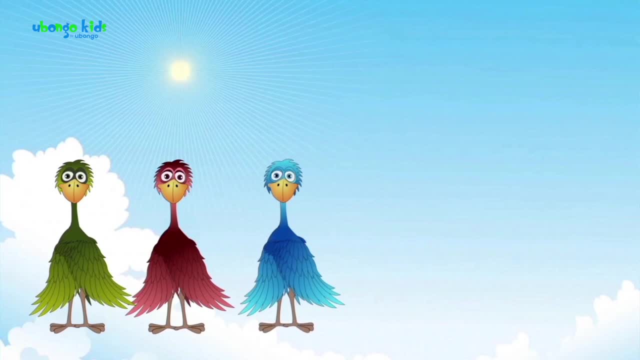 Now look, Gedere. This car has 11 seats And there are four of us here already: Me, pink, blue, How many is that? Three right And the monkey now. So there are four of us plus you, which makes 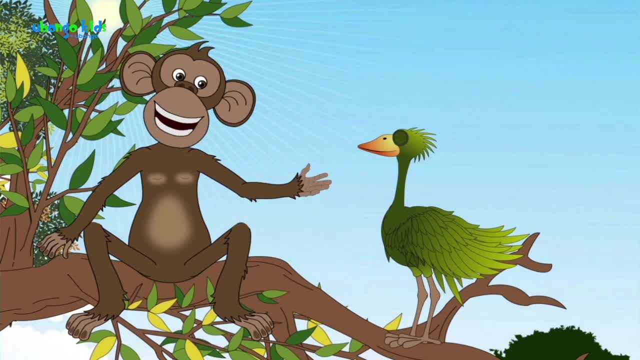 five in total. How many different ways must I explain this to you? We need 11 people: One, two, three, four, five, six, seven, eight, nine, ten, eleven. Now hold on Gedere. We know that we are not enough, But what you need to figure out is how many more passengers 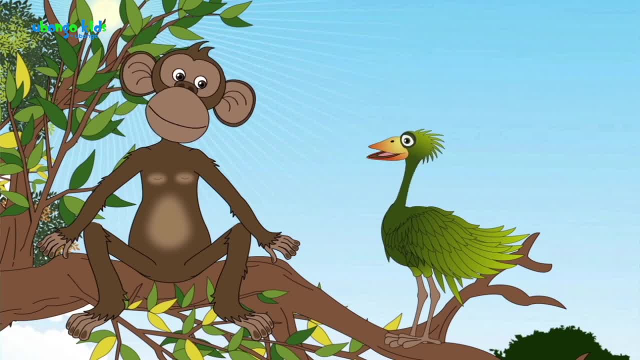 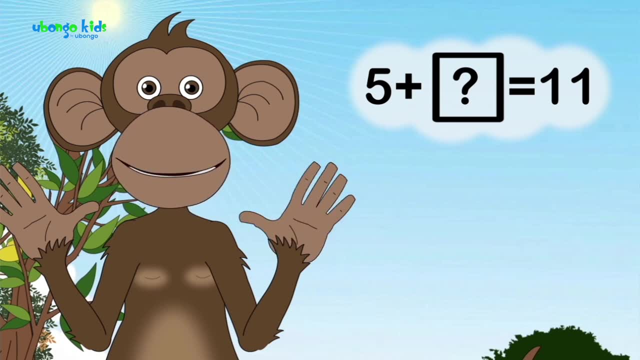 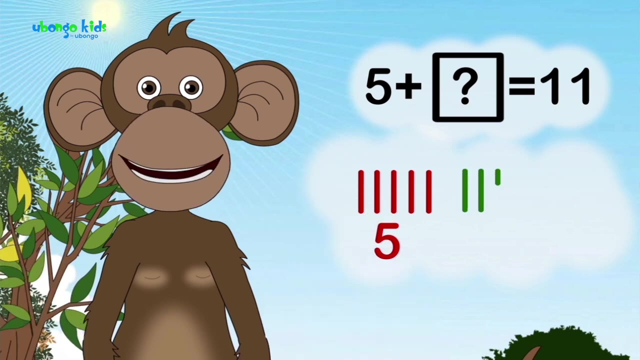 we need to fill it. So let's count up from five to eleven to see how many more you need: Six, seven, eight, nine, ten, eleven. So how many more are left? One, two, three, four, five, six, Oh, okay. 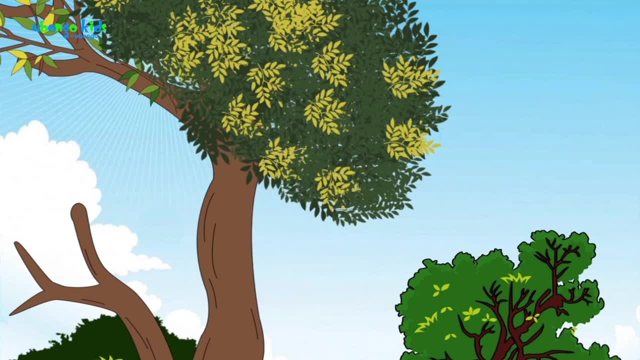 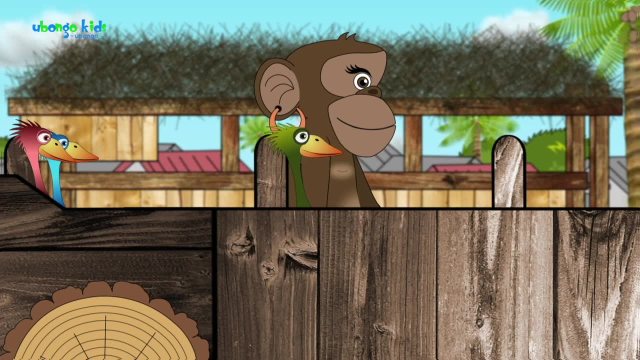 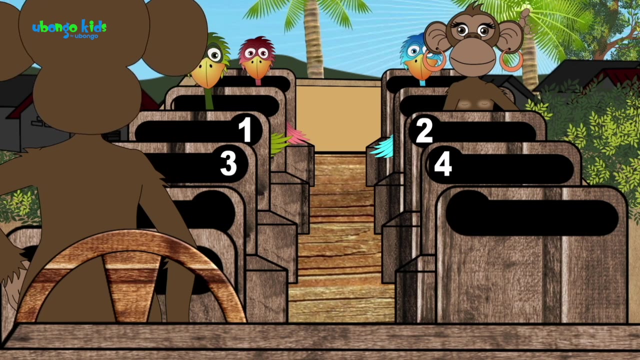 All right, then Come on board. Well, all right, Mama Ndege. Let me count the number of remaining seats and see whether you were right. Okay, then, Good luck with the counting. One, two, three, four, five, six. 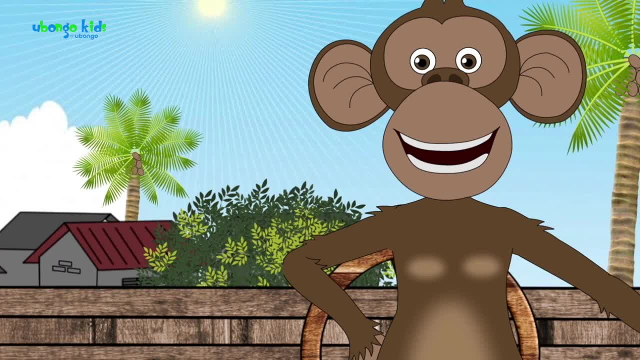 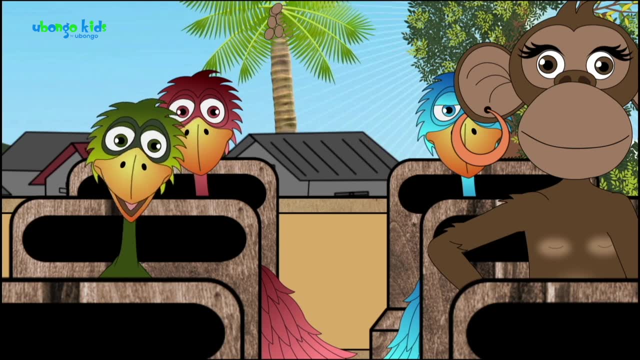 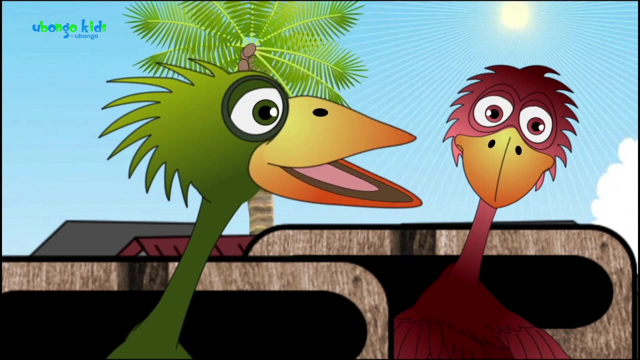 Ah, it really is six. We calculated right. You're a genius, Mama Ndege, And now you know how to calculate the missing seats. What are you all so excited about? It's really no big deal. It's simple math. 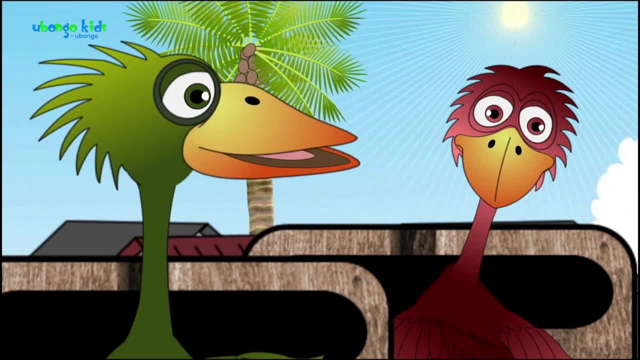 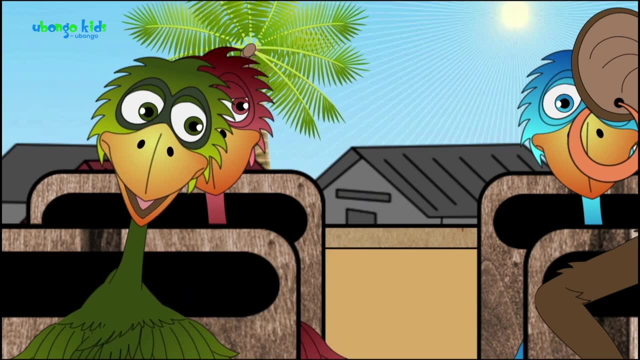 Now it's time to find six more passengers so we can get moving. Okay, one at a time. now We have to count you as you climb on board. There is already five of us on here, So, one by one, you guys come up. 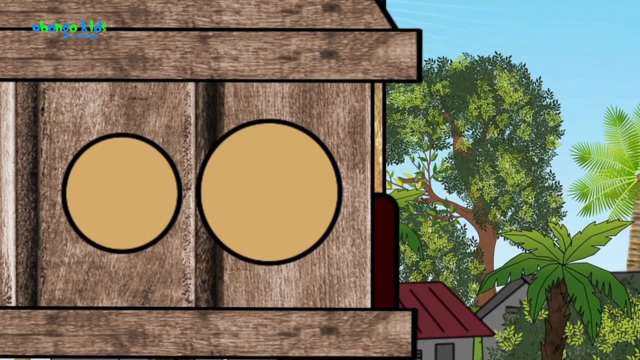 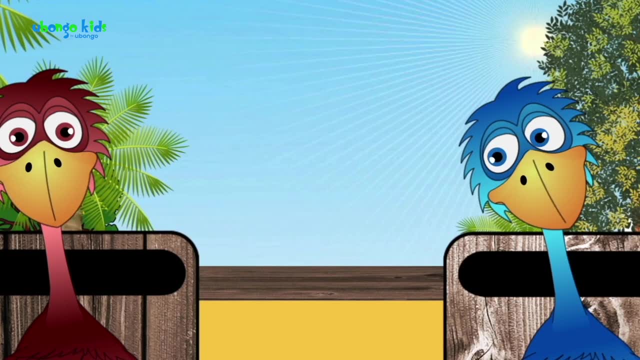 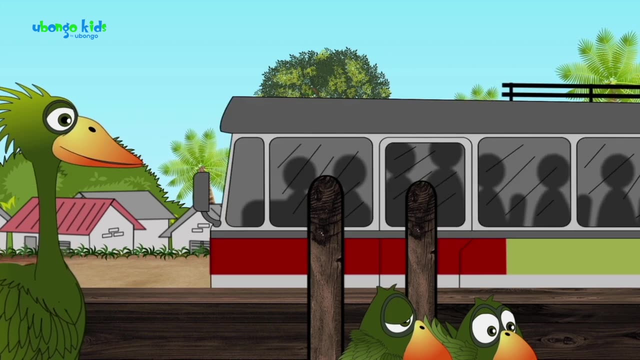 Six, seven, eight, nine, ten, eleven. Thanks, Mama Ndege. Math really has made this easier. Yep definitely has. Hold on Ndege. We've got you two always. Where do you kids think you are going? What are you doing here? 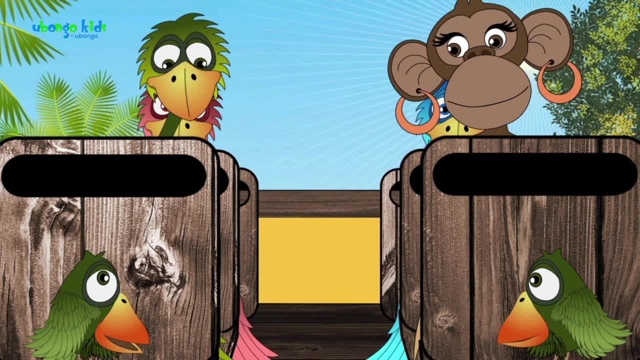 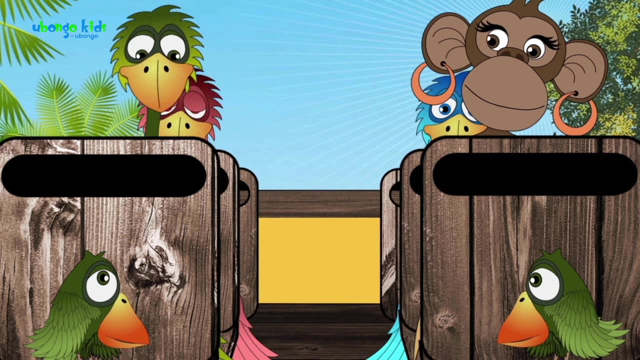 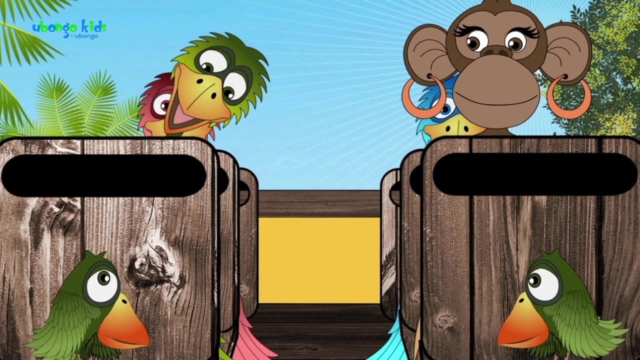 We heard there is a singing competition, so we are going to compete and show how we can sing, just like you, Mommy. Yeah, just like you. We love to learn. Let's learn together. Ah, ah, ah. Let's learn together. 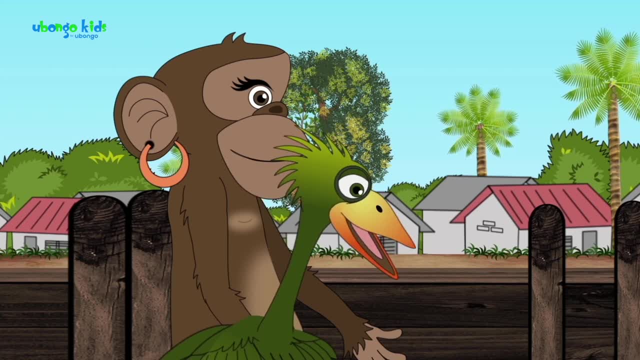 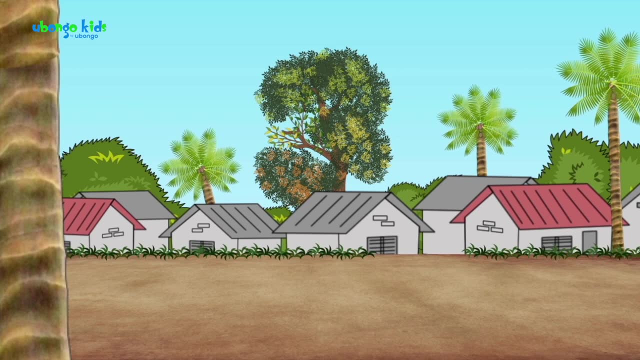 Okay, I have decided You can come, but you need to behave yourselves. No fooling around, We'll behave. Okay, driver, Let's go. Hi everyone, It's good to see you all. How are you doing? 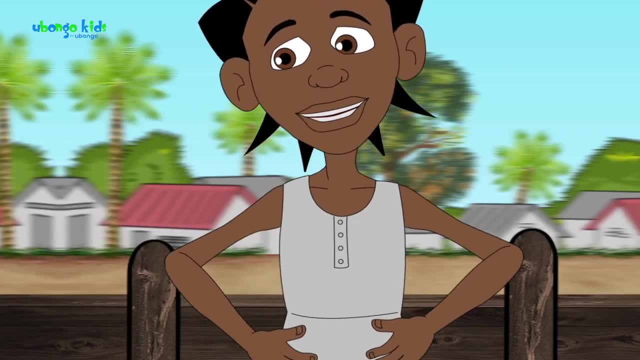 We're good. How are you? You're doing fine, And yourself, Hello, Hello. Do you know that we're the judges for the competition today, You, You and who else? Me, Koba, Baraka and Kiruchu? 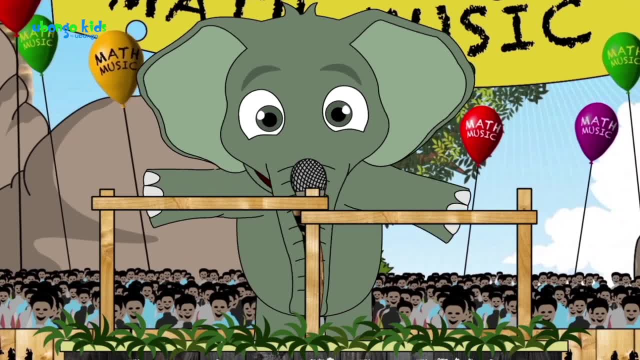 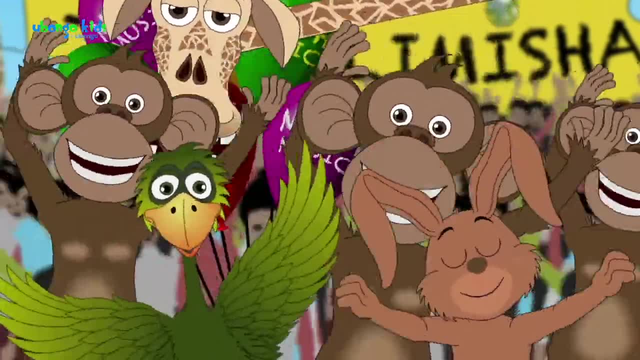 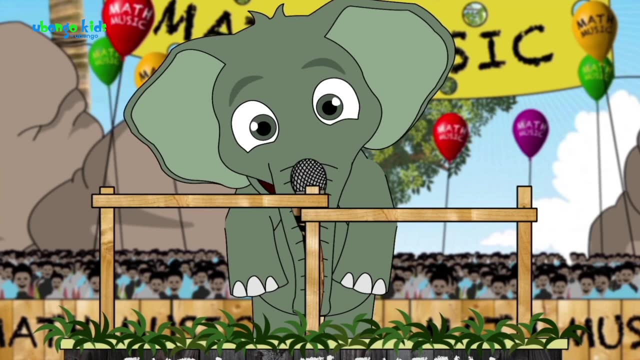 I would like to say welcome, yeah to the special competition. Yeah, come out and sing. The best will win. Yeah, yeah, yeah, I love it. I love it. That was awesome, That was amazing. And the first of our competitors are the Songbird Twins. Yeah, 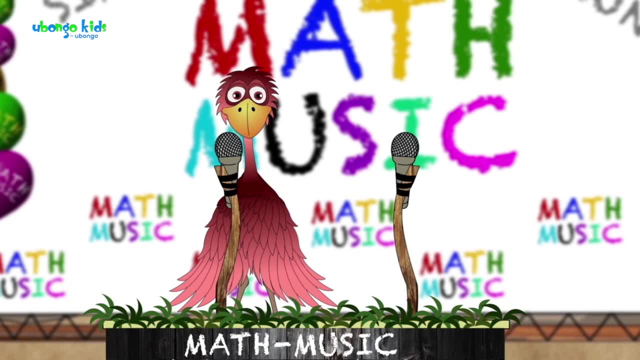 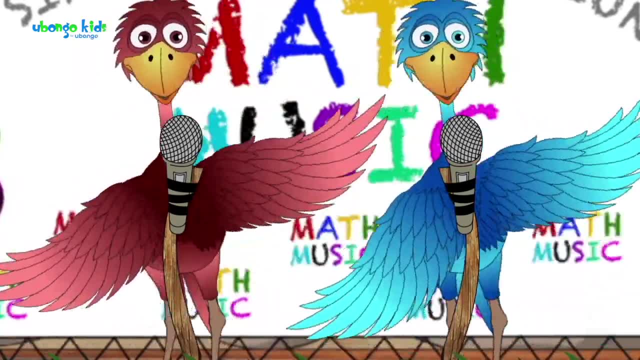 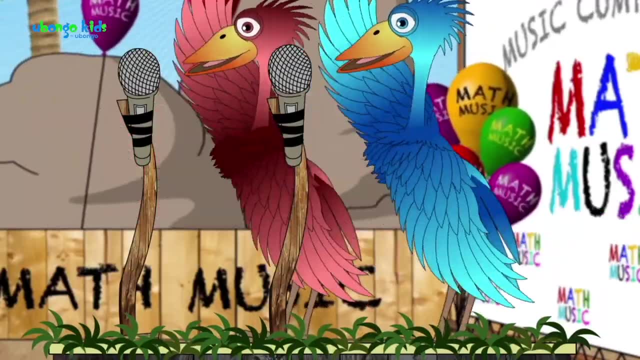 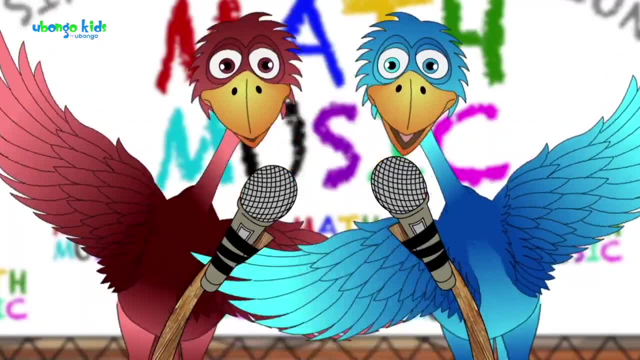 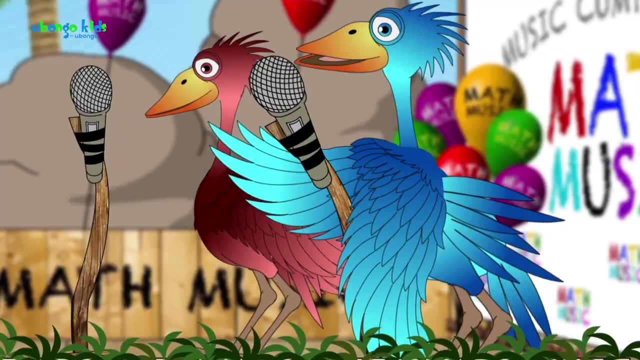 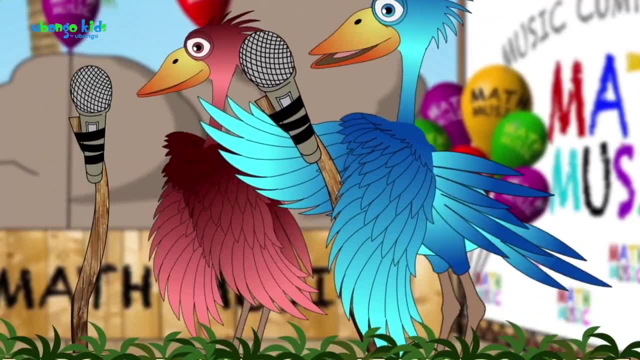 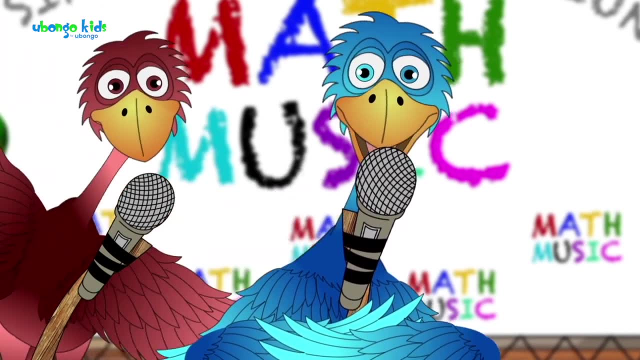 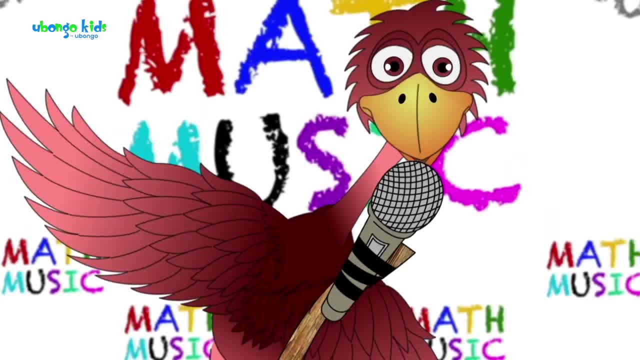 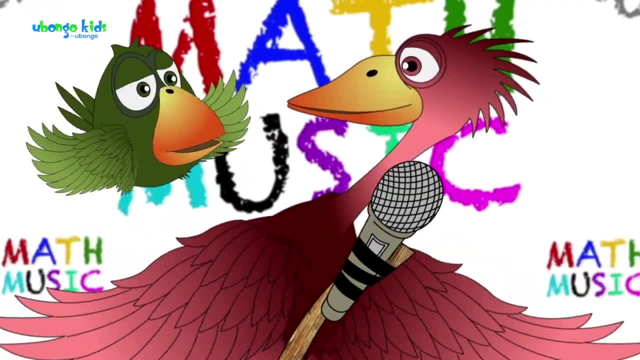 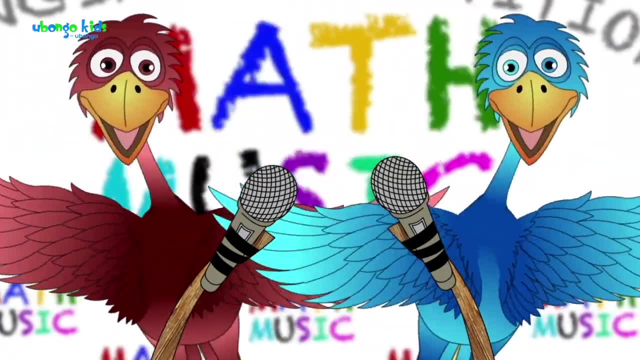 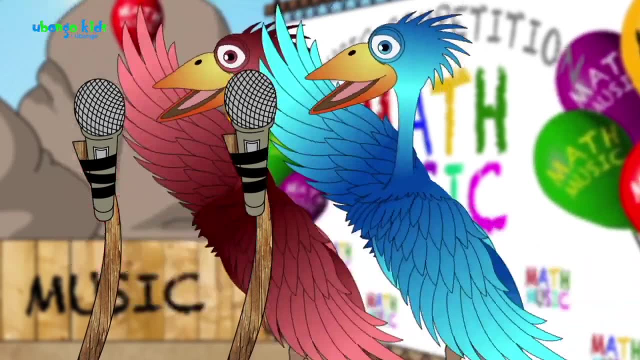 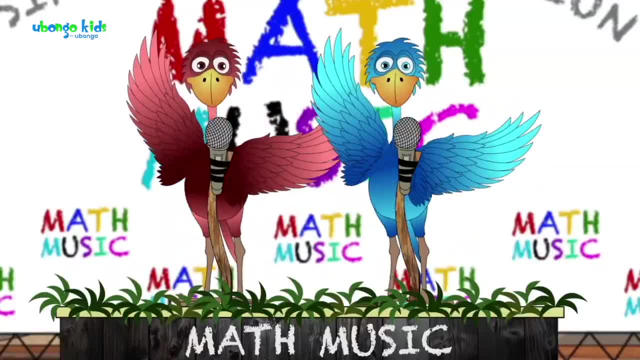 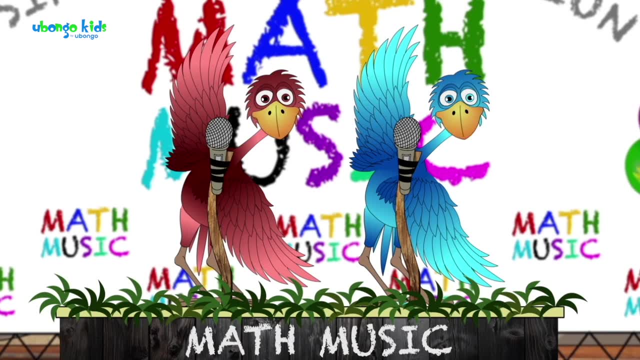 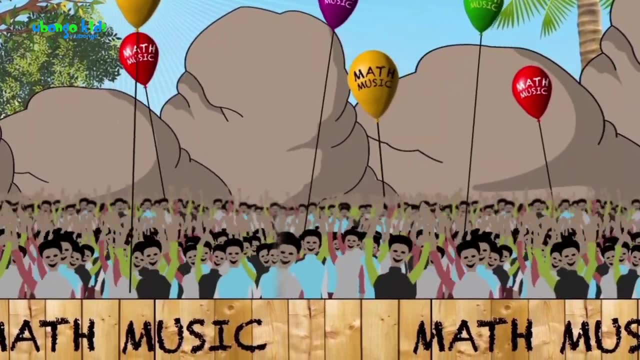 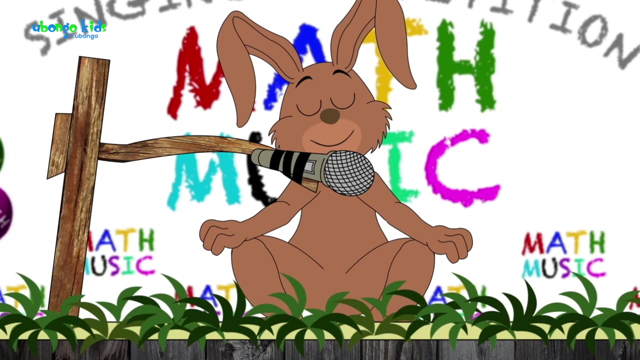 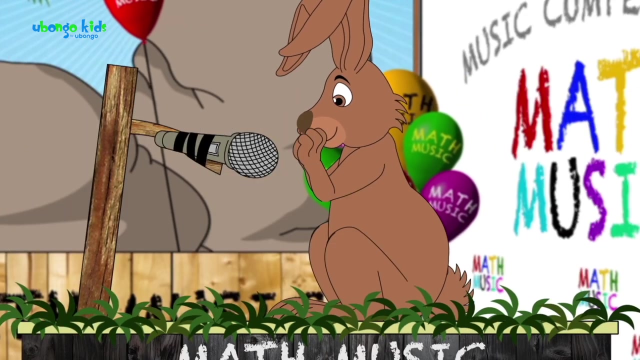 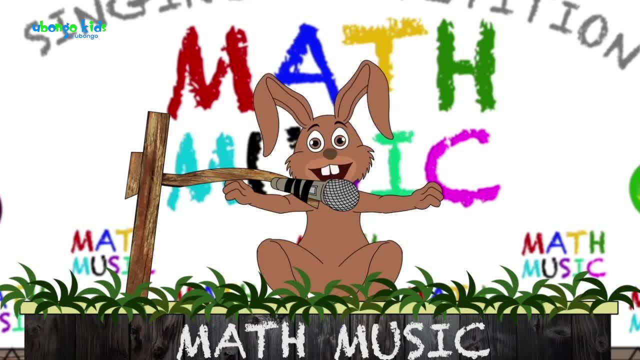 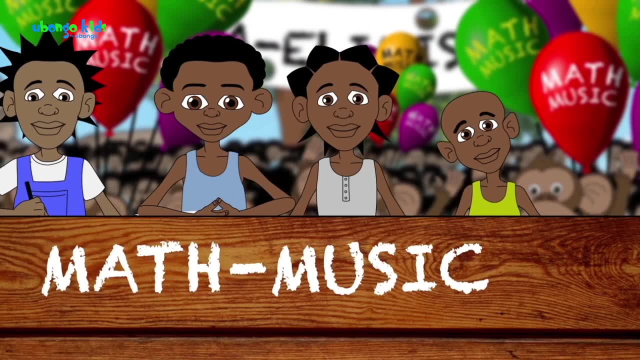 Sorry folks, I have a bit of a sore throat at the moment. Luckily for you, otherwise I wouldn't have won this thing. What have you done? That's a good effort, Tori. Next time, Please no more. This song needs three voices. 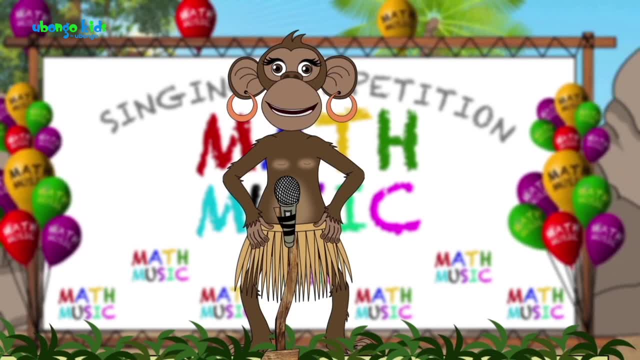 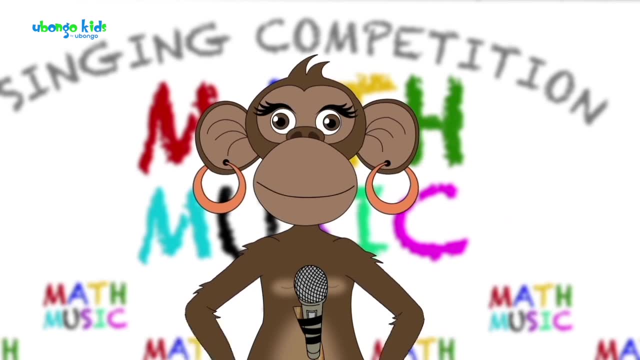 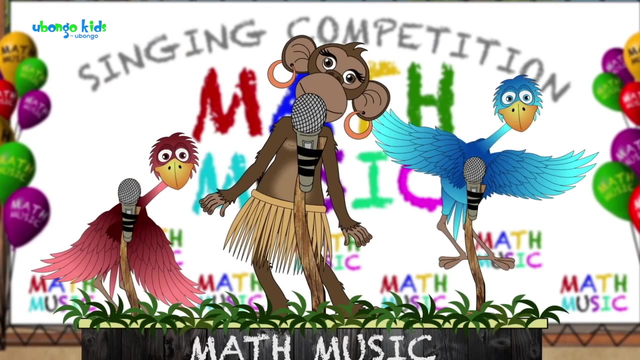 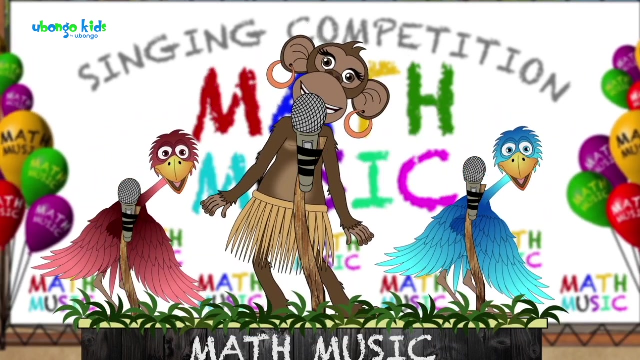 And, as you can all see, there's only one of me, So how many additional singers do I need before I can rock this house? You need two more singers: Alright, Pink and Bluey. why don't you help her out? The mangoes have gone missing. 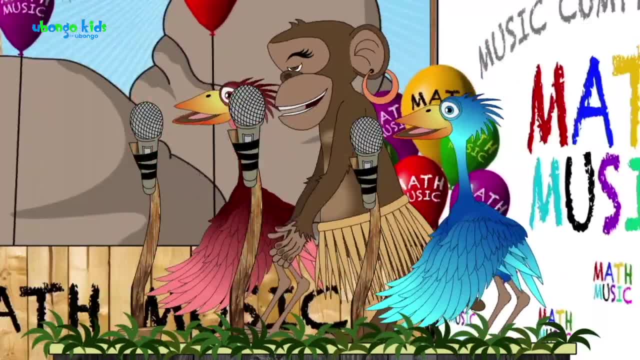 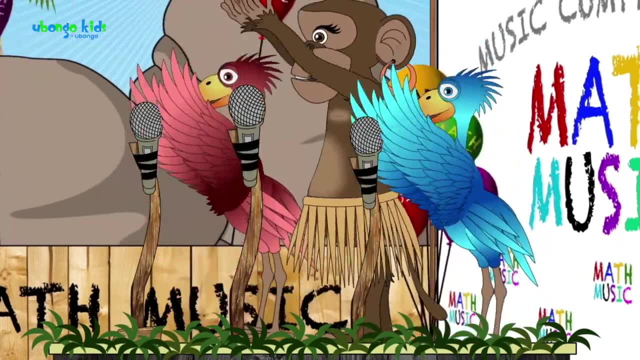 What can we do? The mangoes have gone missing. The mangoes have gone missing. The mangoes have gone missing. What can we do? What can we do? Mangoes are a fruit, a food we love to eat. Now we're so sad cause they're never to be seen. 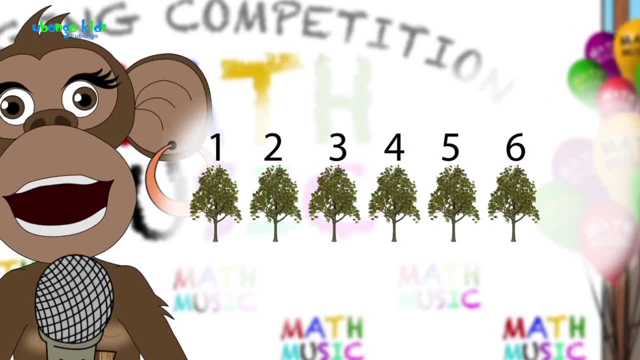 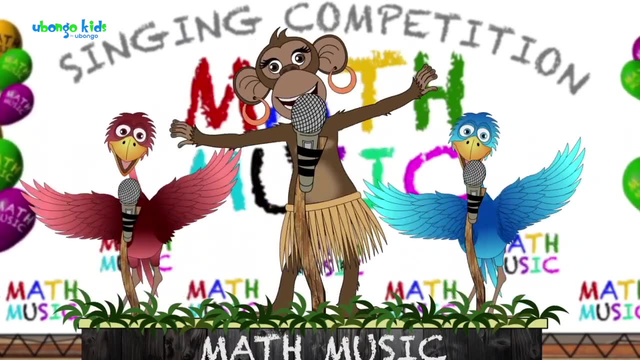 There were seven mangoes and now there are only six. How many mangoes have gone missing? The mangoes have gone missing. The mangoes have gone missing. The mangoes have gone missing. What can we do? What can we do? The mangoes have gone missing. 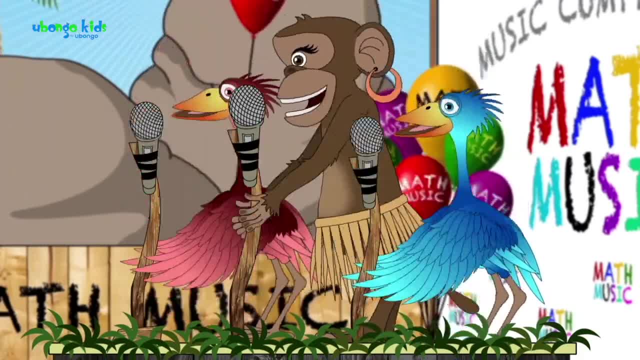 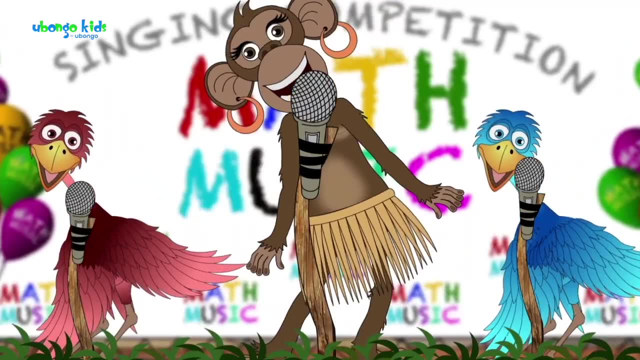 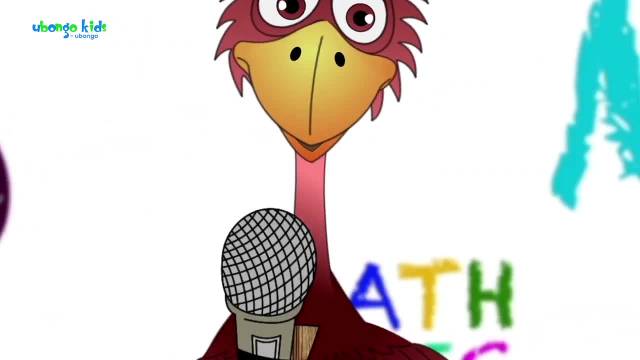 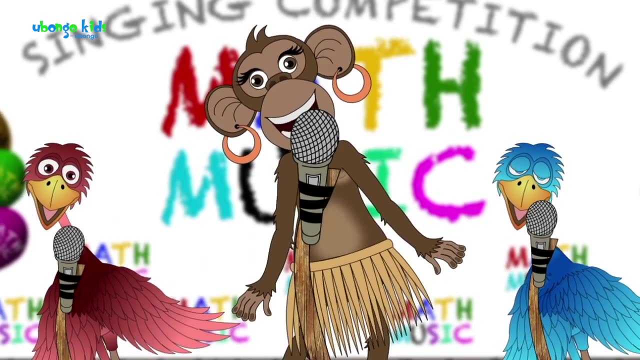 What can we do? What can we do if we're not able to tell what's in their heart? We have to do it, Because if we don't tell it right now, then we want to die. Call your today, call today, Tell it now So you and I can stay a day. 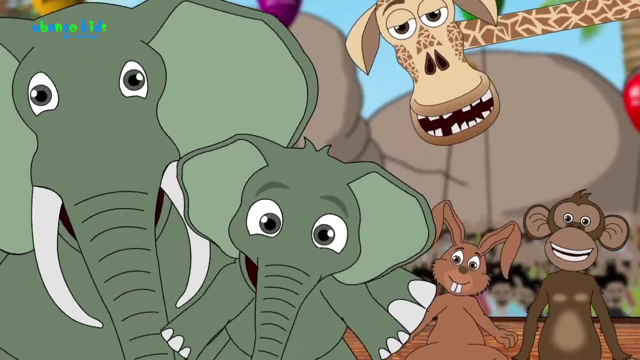 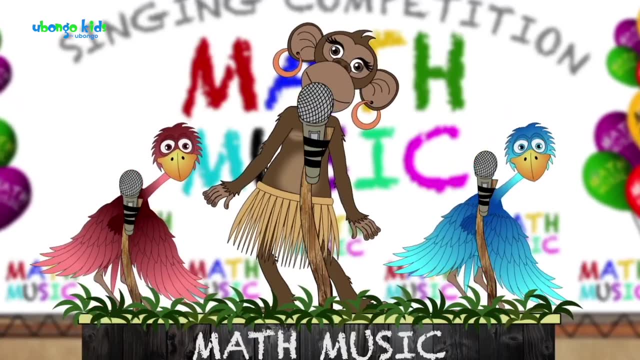 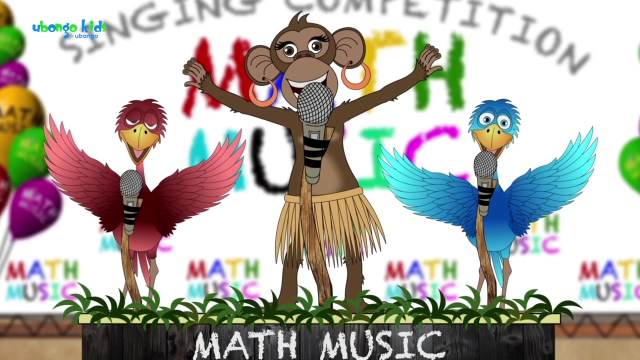 And I can feel the growth in you. 完. And I want Nine's name Go Mark Groove. Fine, Fine, Oh, oh, yeah, yeah, oh oh, I love you, I love you. That wasn't you, it wasn't you. I thought you were singing us. 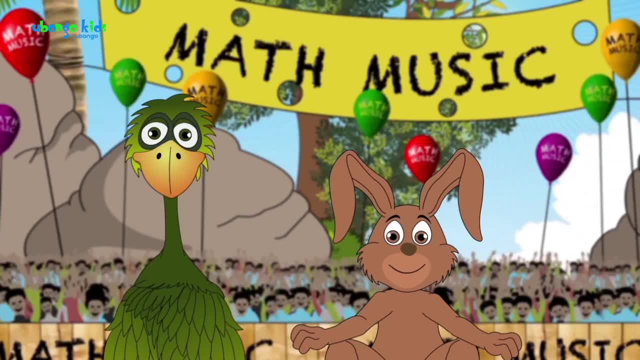 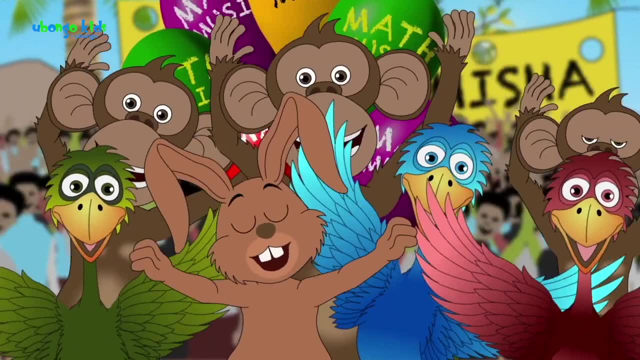 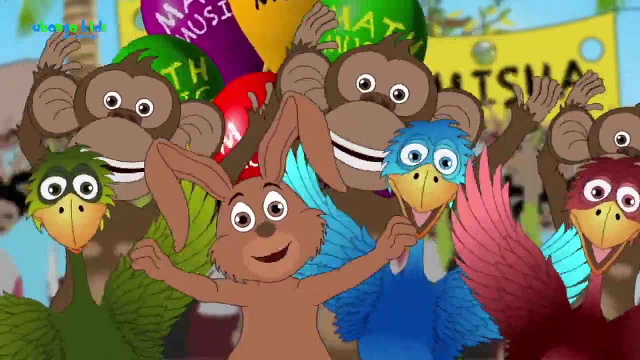 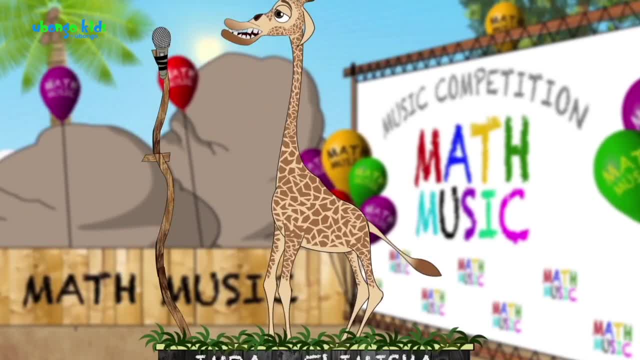 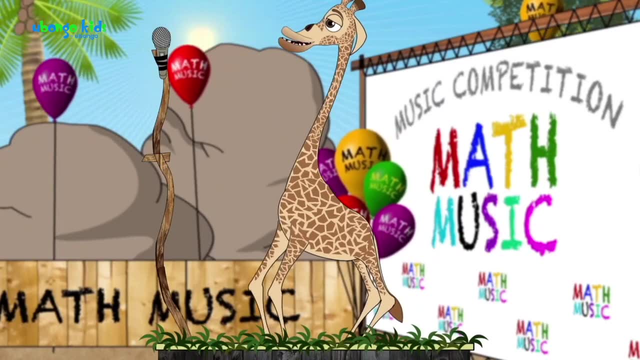 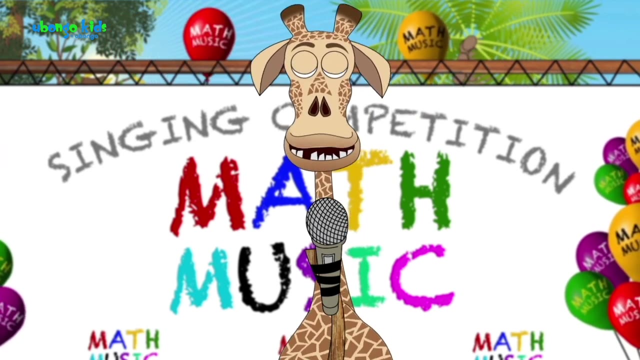 My neck is very long so I can see quite far. I love my math and I'm a rap superstar. Math is like music to my ears. Numbers are simple. there's no reason to fear What's up. kids Listen to me, and you must listen hard. 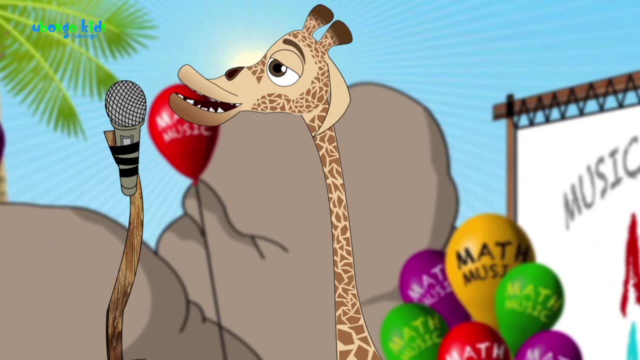 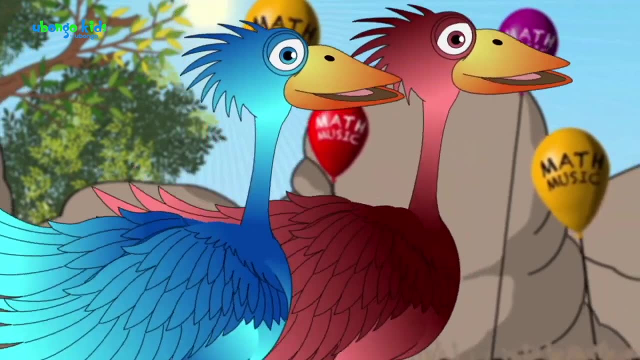 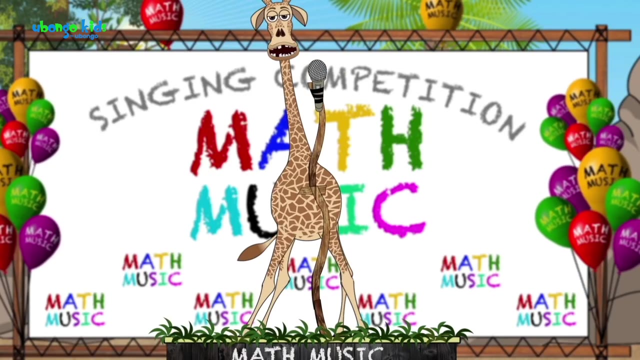 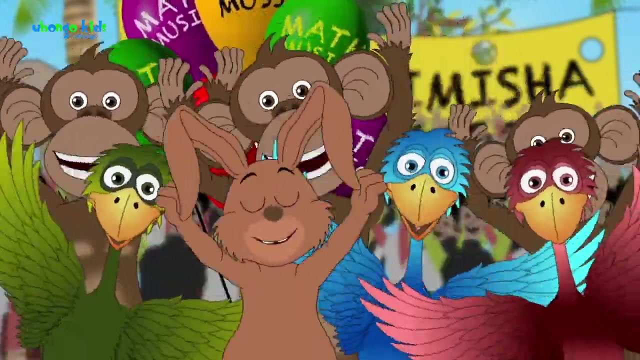 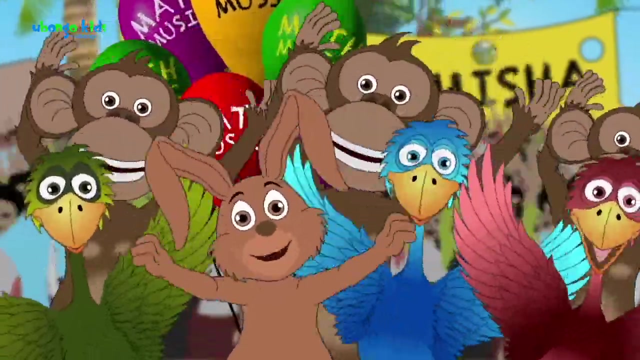 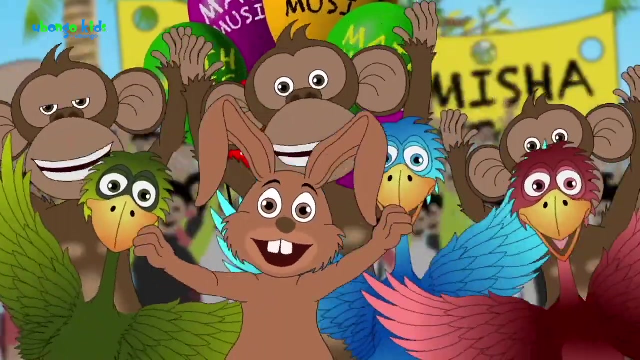 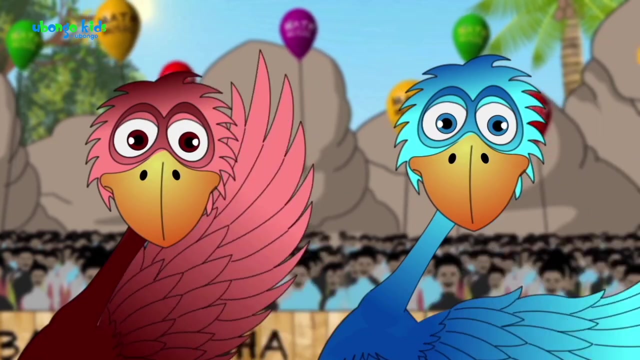 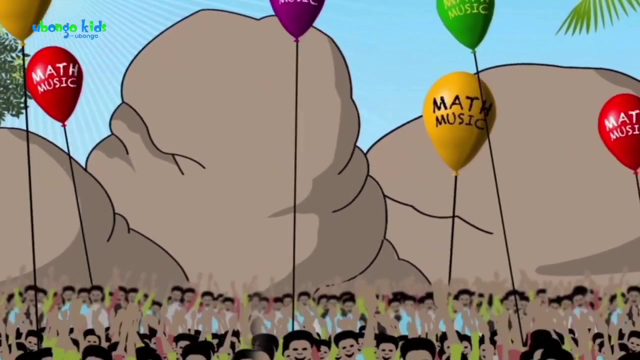 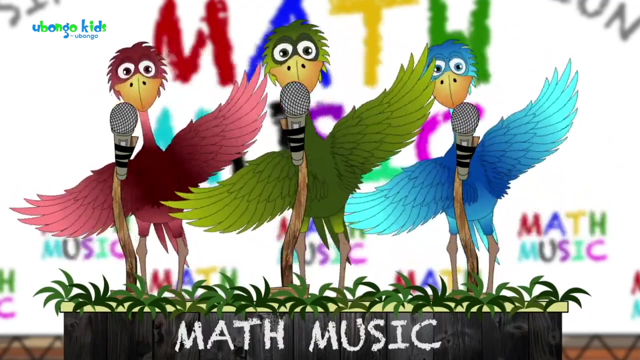 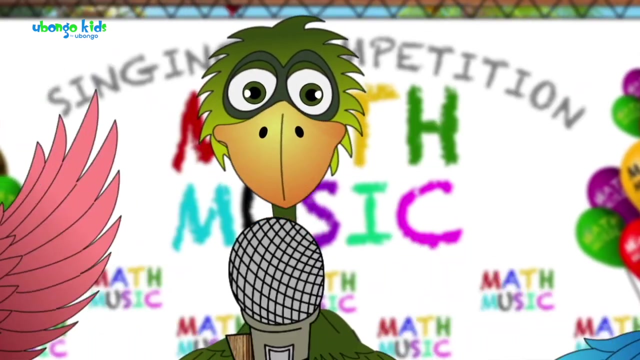 Trust in math and you'll go so far. Hey kids, what I say is true: Math will always be true. Open noodles for you. I'm Gucci, I'm Gucci, I'm Gucci, Thank you. Money remains undiscovered. Once it becomes known, then it is uncovered. 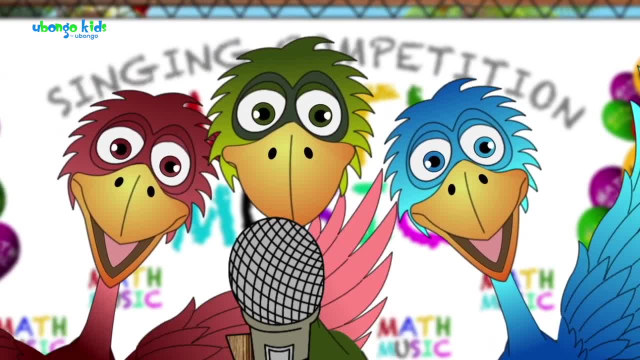 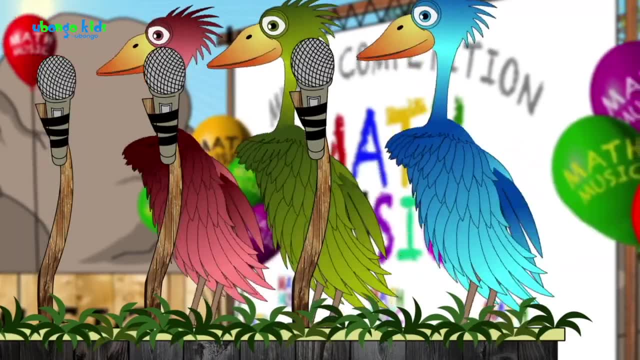 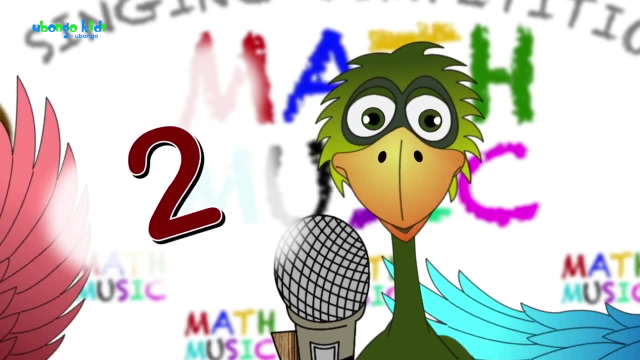 So get questioning. yeah, Mathematics can help with answers that you need to find Numerical problems unraveled by your mind. When you see the number two, you should start to question: Two is a number, two is a symbol Two. 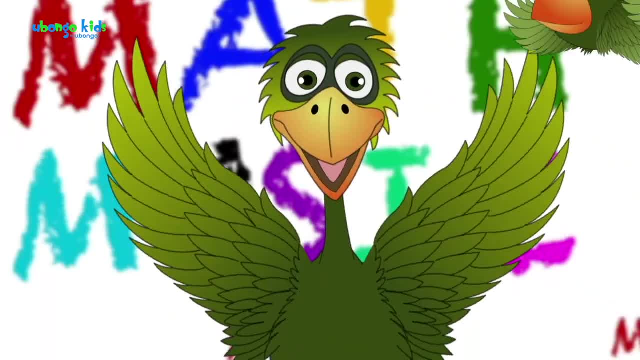 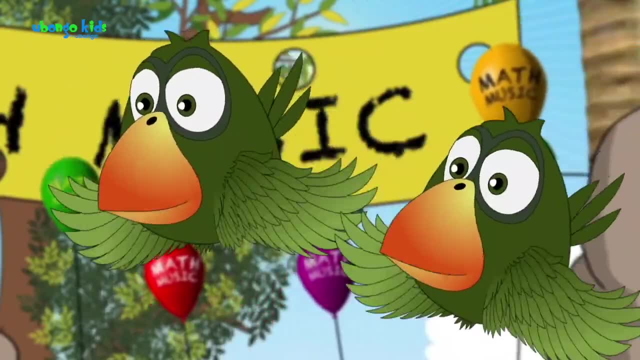 Eyes, too wings, too legs. Ah, and those are my two kids. Ha ha, ha, ha, ha. sing it: kids, Ba ba ba ba ba ti ru ti ru. Ha Ba ba ba ba ba ti ru ti ru. 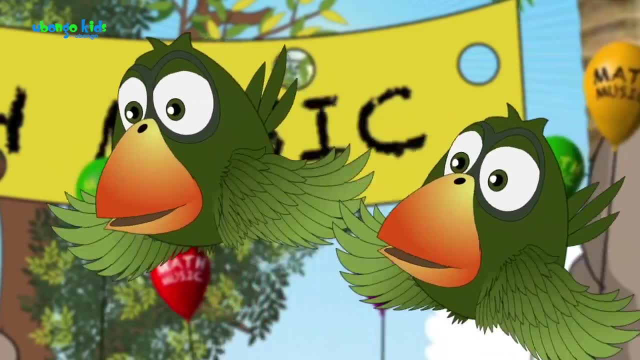 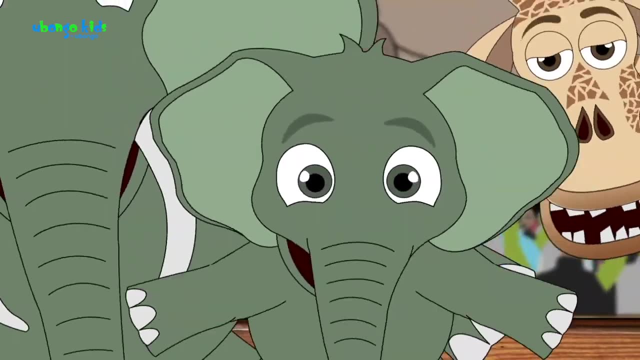 Those are my two kids singing now. Ha Ba ba ba ba ba ti ru ti ru. When you finish the caper: Ba ba ba ba ba ti ru ti ru. Ha Ba ba ba ba ba ti ru ti ru. 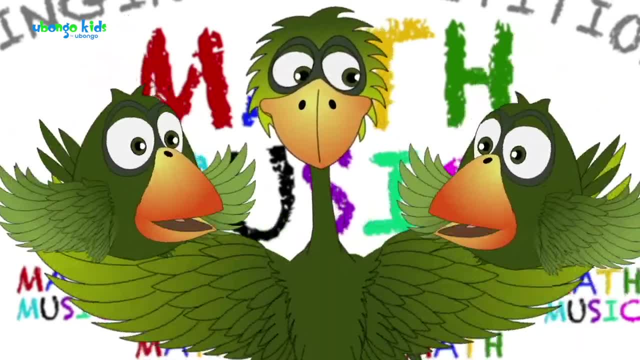 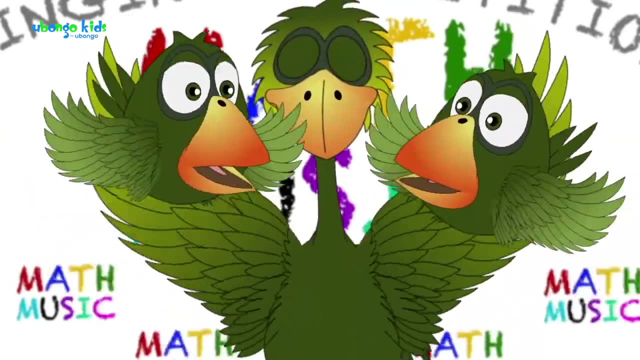 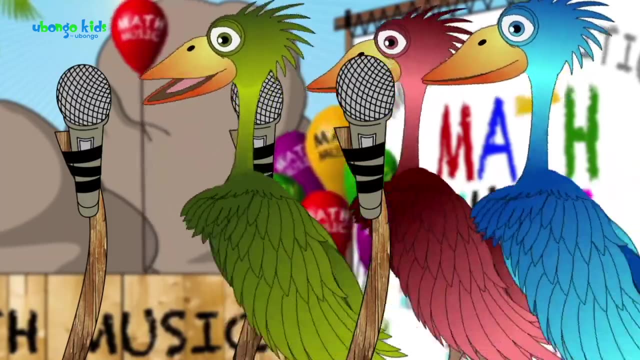 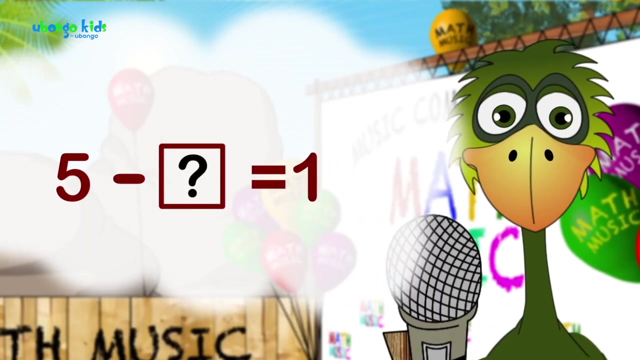 Ba ba ba ba ba ti ru ti ru. Ha ha Ba ba ba ba ba ti ru ti ru. If you were given five hats and you only want one, how many will you have to give away? Now, there is a number there that is missing. that will give you. 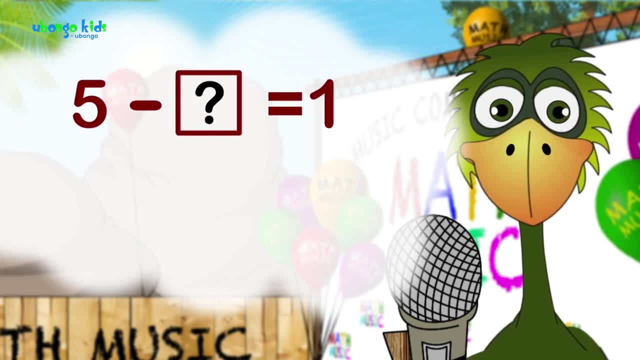 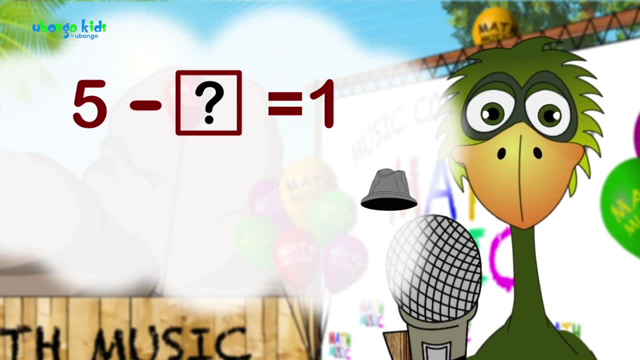 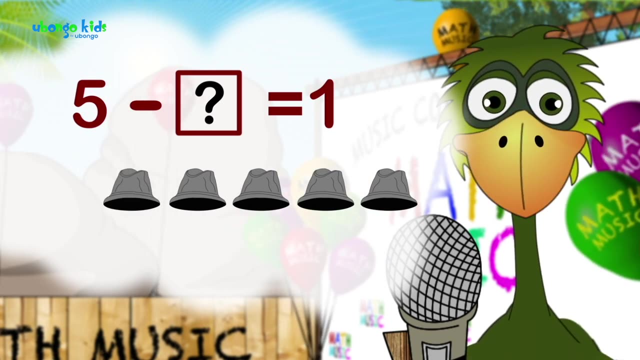 an answer of one. You know that number, You know the number. you see. Tell you what. why don't you give me five hearts: One, two, three, four, five? You see the five hearts. I only want one. 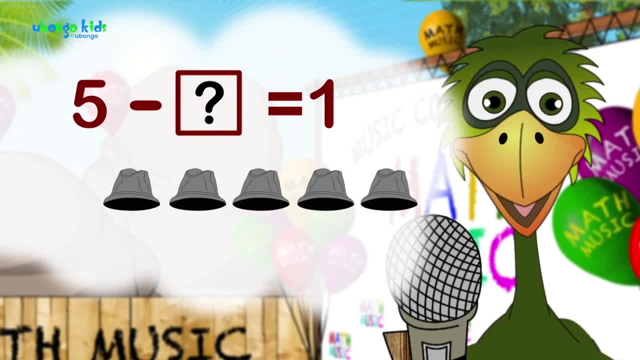 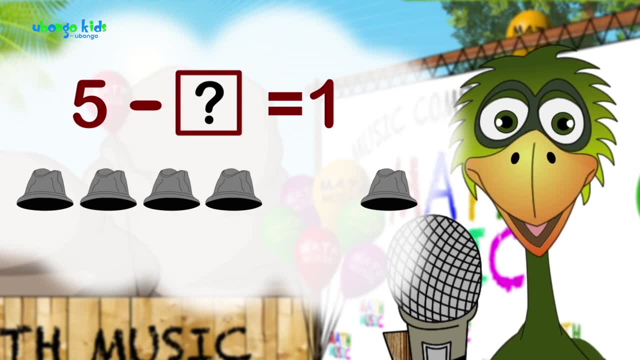 How many should I give away? That number is what we are seeking. the missing number: Watch. I am giving away all of the hearts so that I remain with one, you see. So the missing number here was four. What's five minus four? 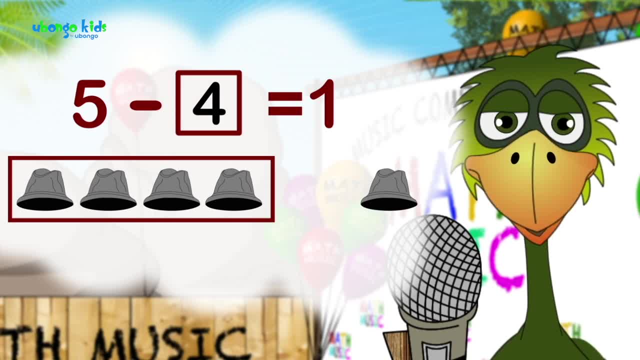 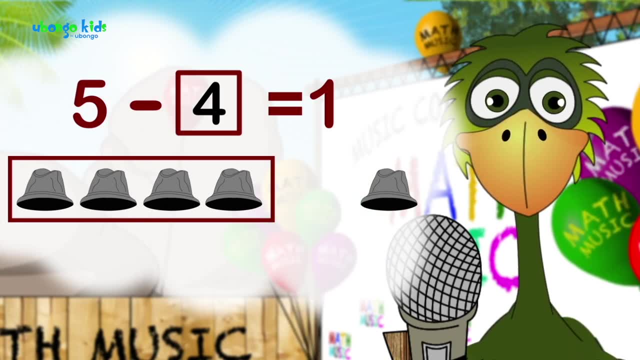 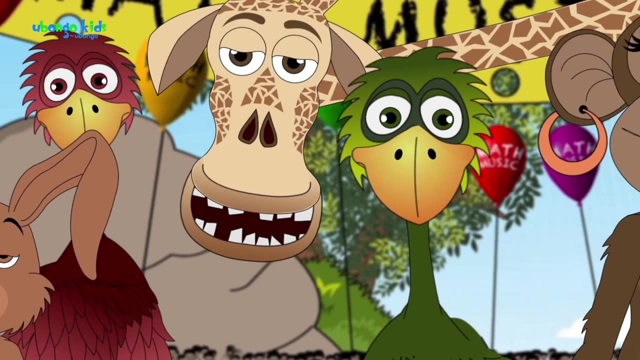 Come on, guys, you know this one. Don't wait for me to answer it for you all the time. Thank you to all the competitors and the amazing crowd. Now it's time to announce the winners: Husangwo and Explodewell. 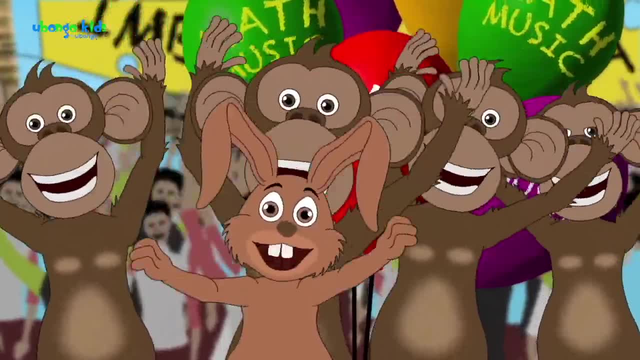 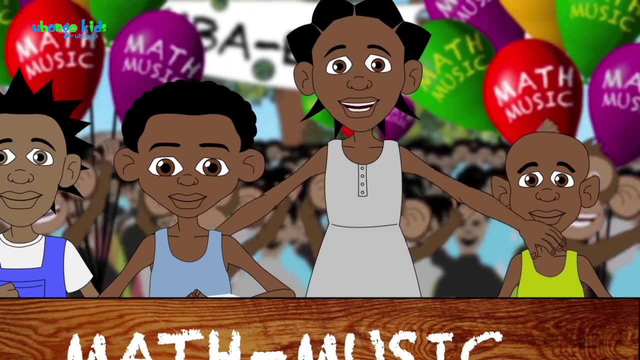 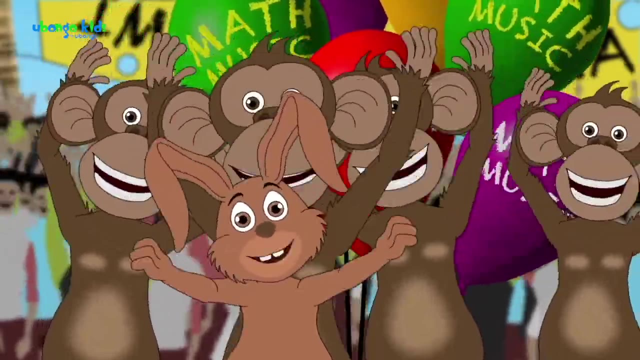 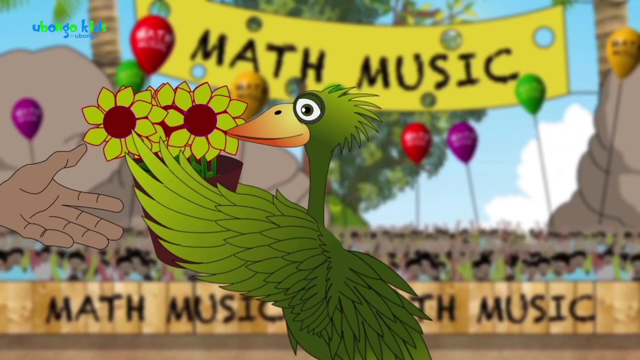 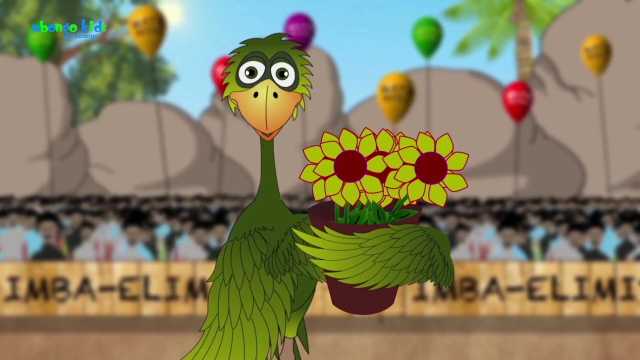 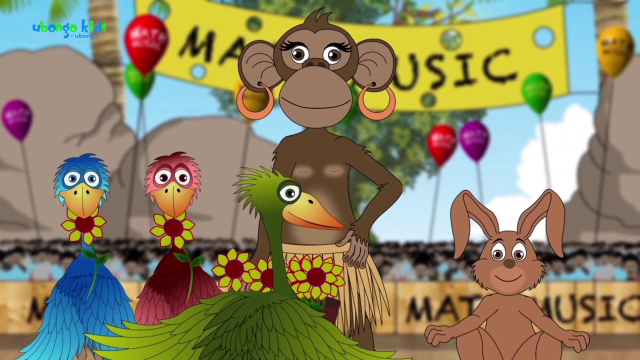 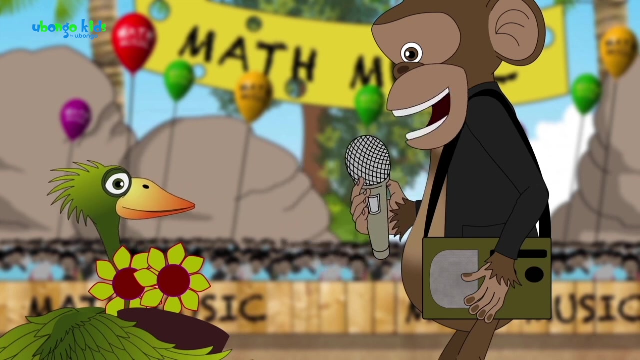 The winner is Mama and Zagat. Oh man, Thank you so, so much, But everyone is Everyone is, Everyone is Everyone. here is a winner. Congratulations, Mama Ndege. Thank you, I'm Gedere from Kokotua Times. 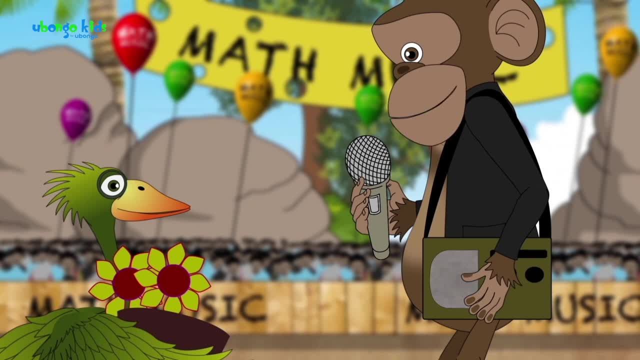 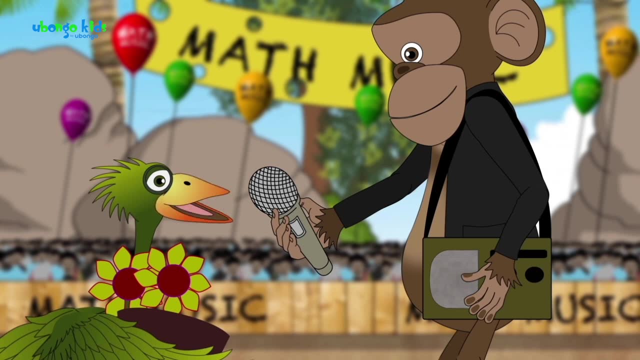 Tell us how many flowers were in the prize this year. Oh no, I didn't even count them. I gave five flowers to each of the other five competitors And I have two left here. Let me ask you a question. Are you ready? 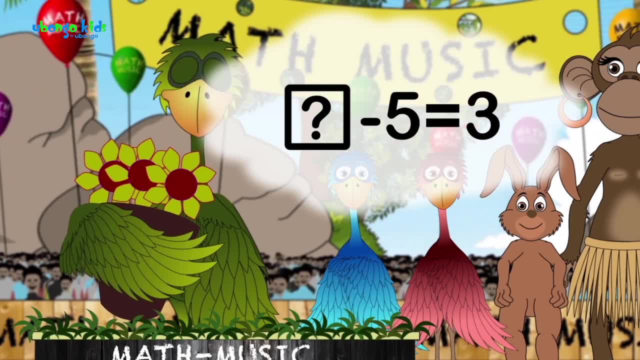 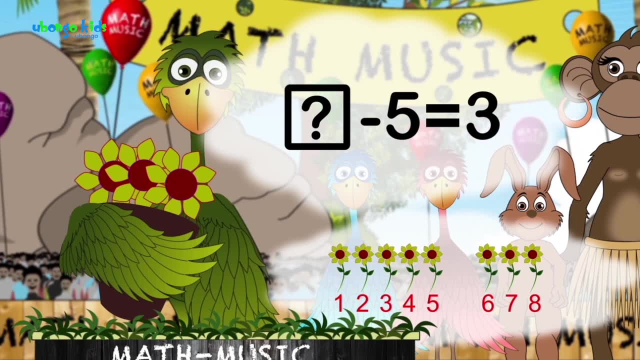 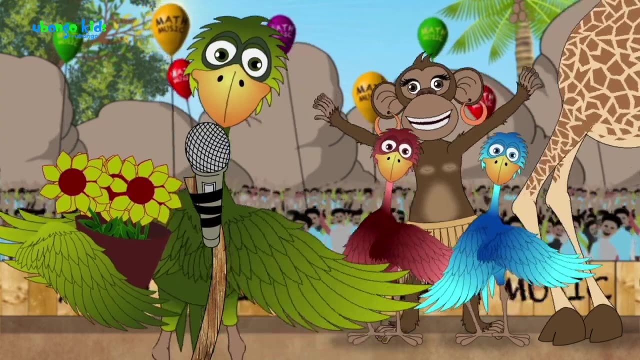 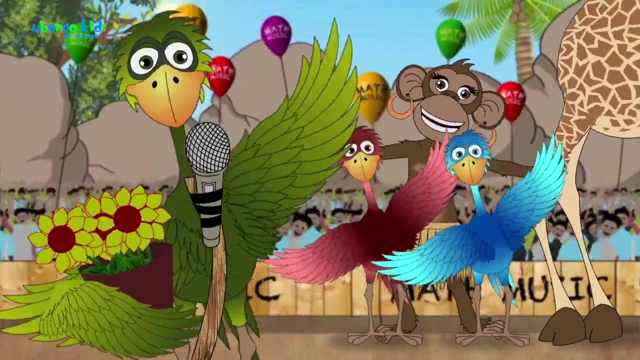 What minus five equals three. Now I gave out five and I'm left with three, So in total there were eight flowers. Well, congratulations, Thank you, Thank you, Thank you. And no, it remains undiscovered. 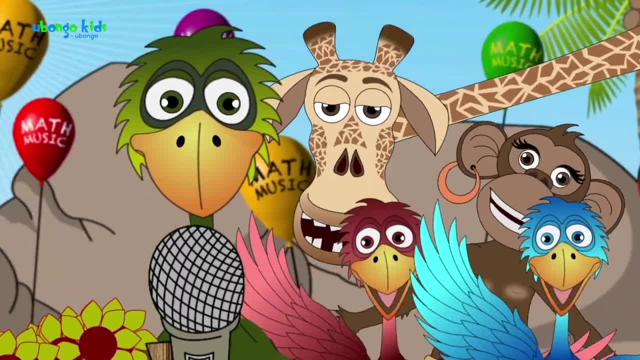 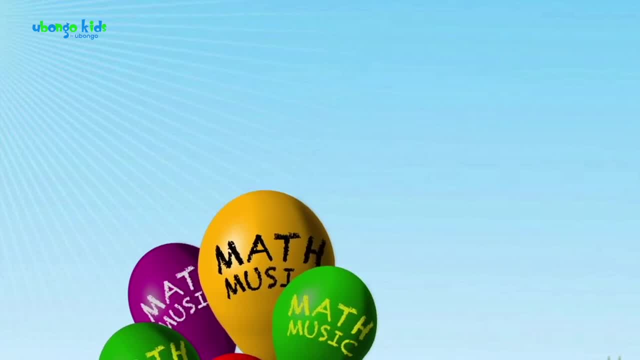 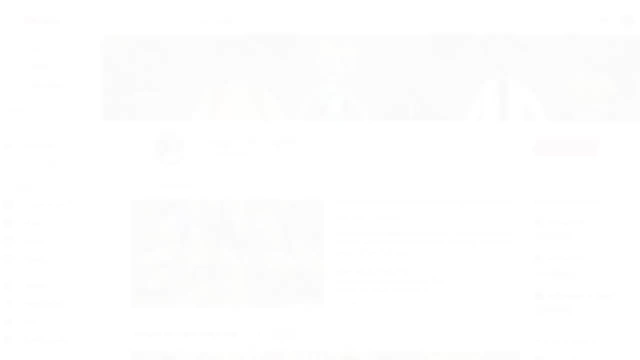 Once it becomes known, then it is uncovered. So get questioning. yeah, Mathematics can help with answers that you need to find, And there the problems unravel by your mind. Never miss out on new Ubaldo Kids videos ever again. 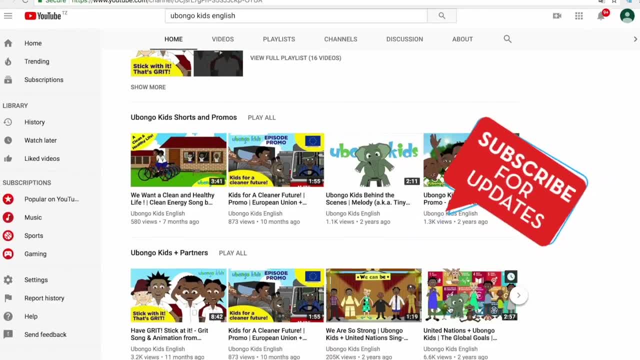 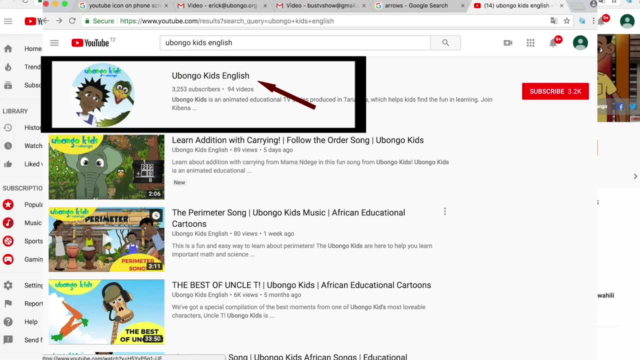 Subscribe today and become the first to know every time new fun educational content is available. Subscribe today and become the first to know every time new fun educational content is available. Simply type Obonga Kids English on the search bar. click on the Obonga Kids English channel page. 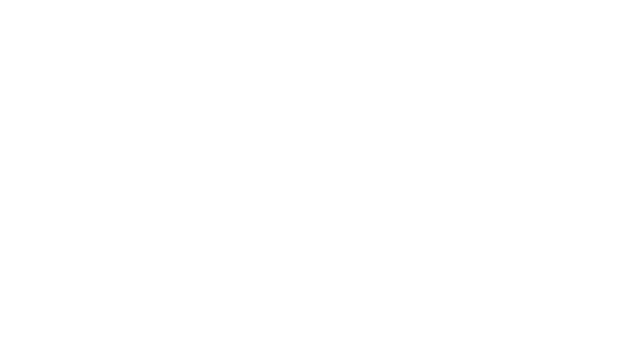 click subscribe on the right-hand corner of your screen. What are you waiting for? You are three easy steps away from joining the Obonga Kids family. 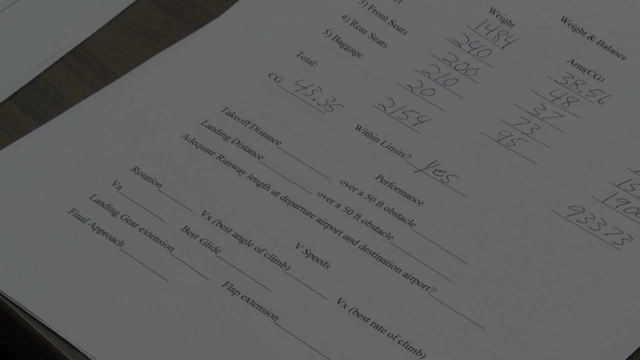 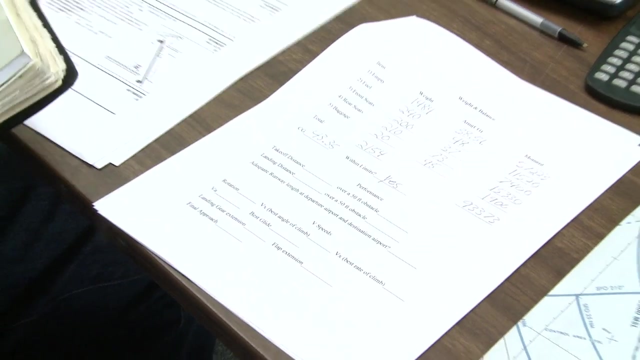 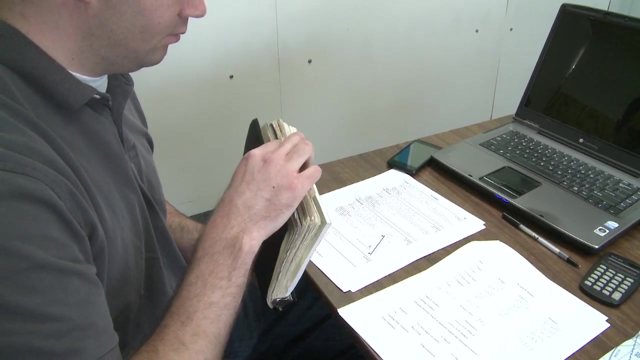 Next, we want to take a look at our takeoff and landing distance and determine if we have enough runway at these airports to take off and land. So for this we need the pilot's operating handbook. We need to take a look at the performance section. Here's the performance. 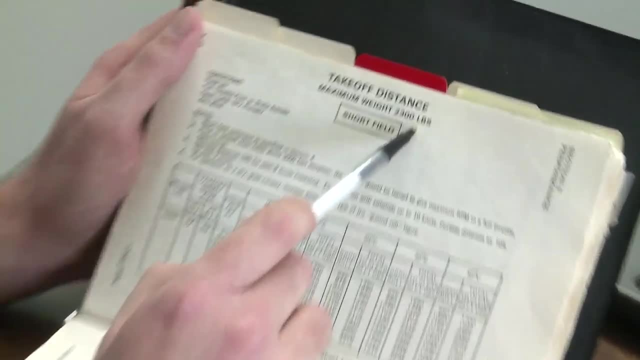 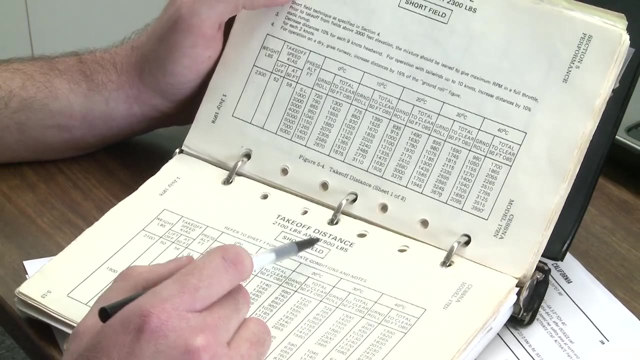 section. This is takeoff distance at maximum weight of 2,300 pounds. Here's takeoff distance at 2,100 pounds and 1,900 pounds. We're closest to 2,100 pounds, so I'll go ahead and use. 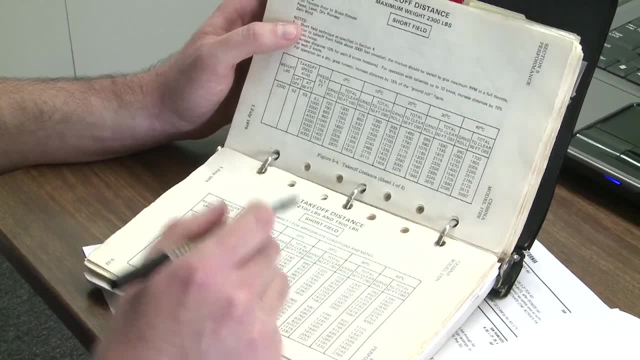 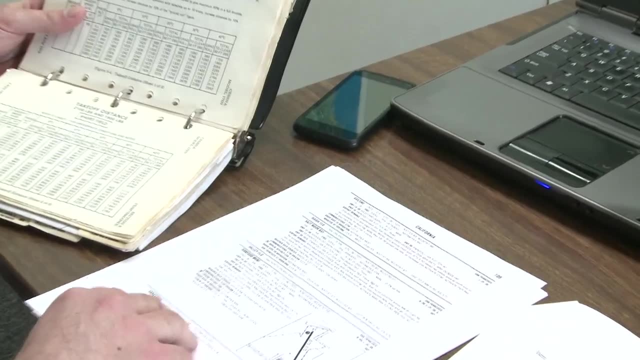 that one. As you can see, it needs a temperature. So how do we determine what the temperature is? Well, if we look in the airport facility directory, there's a phone number in which we can listen to ATIS. So if we look right here, ATIS is on 125.2.. The phone number: 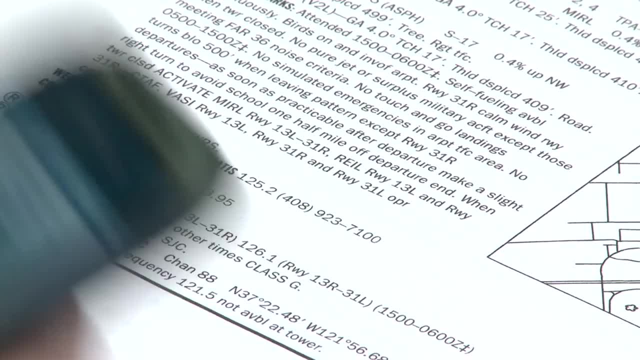 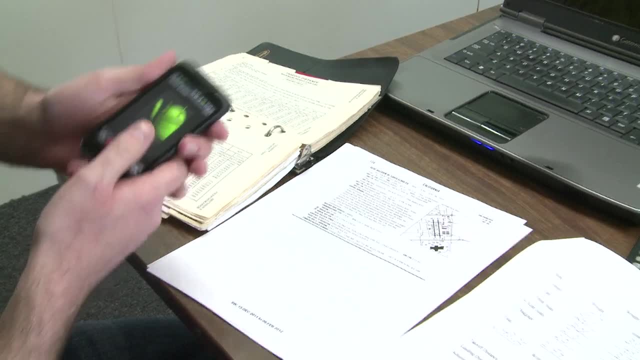 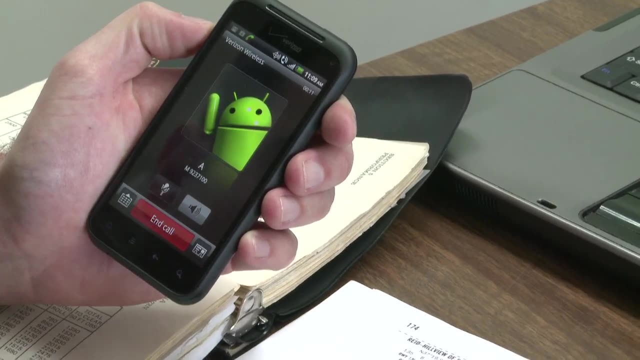 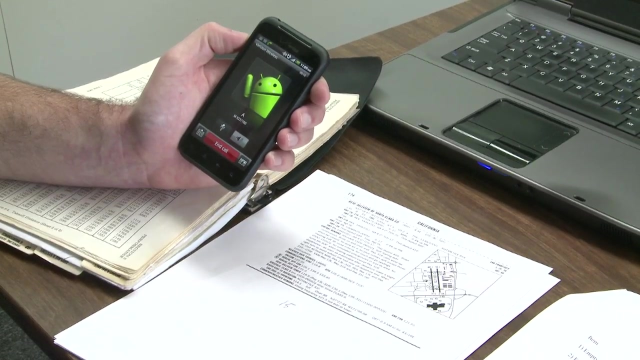 is 408-923-7100.. 0. 28,000 scattered. Temperature: 15.. 2.4.. Altimeter: 3010.. RNAD GPS runway 31 right approach in use. Landing and departing runway 31 right and 31 left. All departures advise grab control.